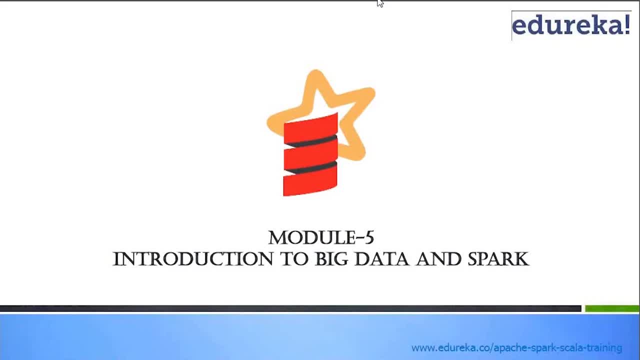 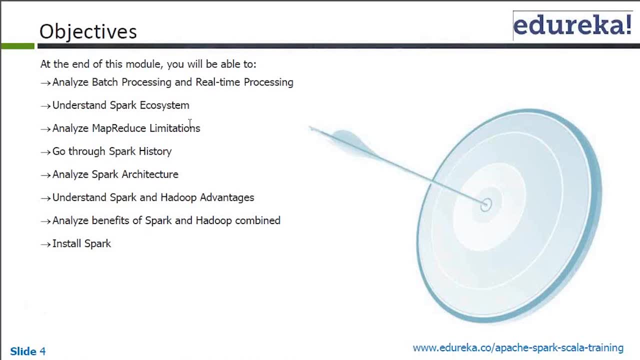 Let's take a bit deep dive into the SPARC ecosystem, what exactly it is and things like that. There are so many people who are not from Hadoop background and all, so there would be some of the primers which are supposed to be given. 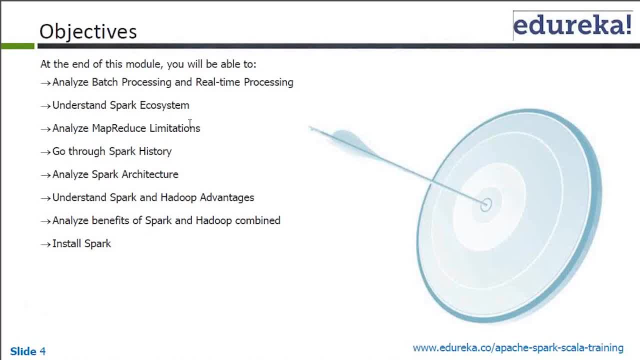 In the first class. we have talked about big data and other stuff. We're not going to spend that much time here, But SPARC, which was seen at a very, very high level, now is the time when we'll start, you know, putting some more in-depth time onto it, right? 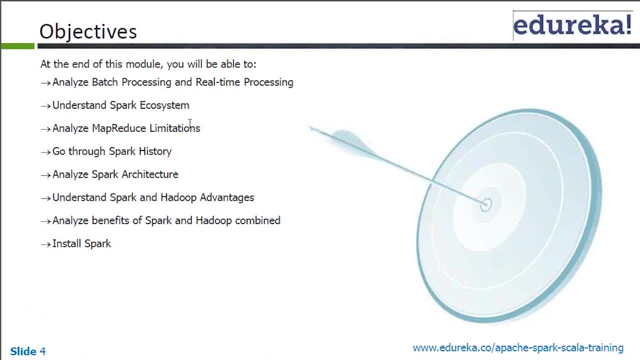 So it works and all. Again, I'm not putting much of the effort into this Introduction to big data in SPARC. Okay so the objects, the objectives which we have had about it in under, So I would try to cover as much as possible in under. you know some 40 minutes or so about batch processing and real-time processing. 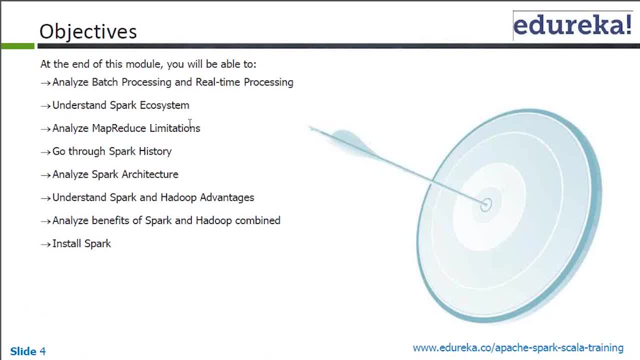 When you talk about batch processing and real-time processing. I am sure if I ask the class, most of you will say yes, we are aware of it. right, But in big data world they have got a slightly different meaning, They have got slightly different scenario and the moment you talk about that slightly different thing. 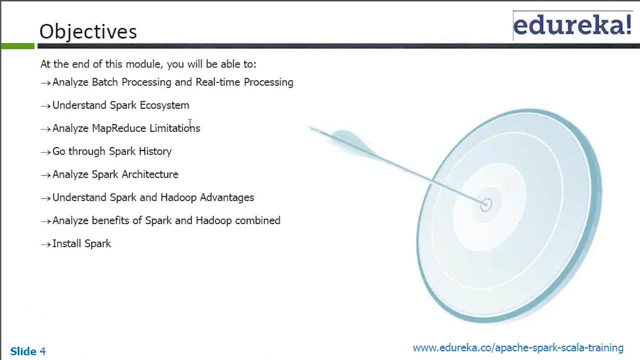 the kind of solution which you are trying to put In fact, so in the last class, I was having discussion with some architects and all wherein the discussion was about that. okay, Vishal, you are telling us that where we should use SPARC. 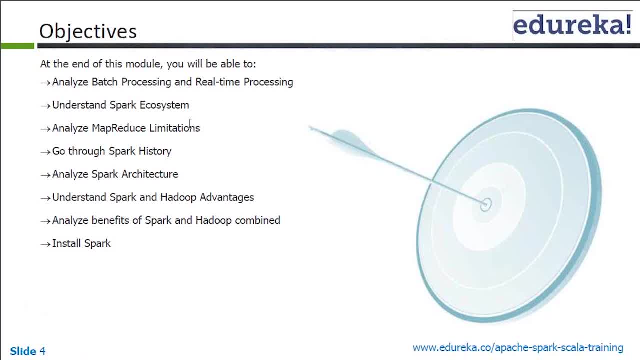 but then there might be, you know, 10 different objects, 10 different other things where you might not like to use SPARC. Right, guys? I hope everybody understands the aspect of it or the implications of it as well, right? 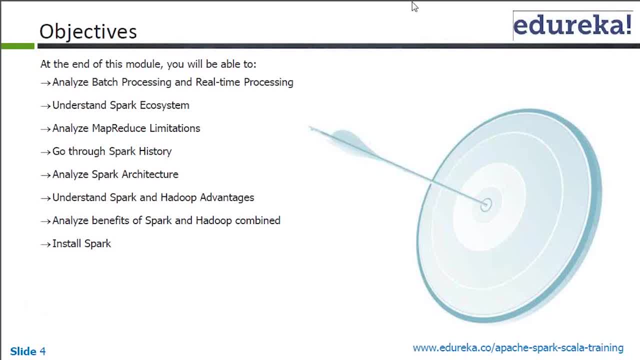 That when you should use, you should know, But when you should not use, you should equally. It is equally important as well, right? So we will see some of those things here. I mean, these kind of discussions are not really written here. 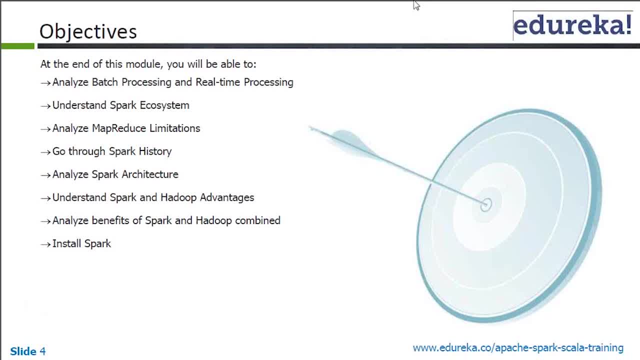 But yes, they would come out right, And then understanding of the SPARC ecosystem in a bit more detail, Understanding of MapReduce limitations themselves. So it is very important. I mean a bit. It would be a bit history kind of a thing. 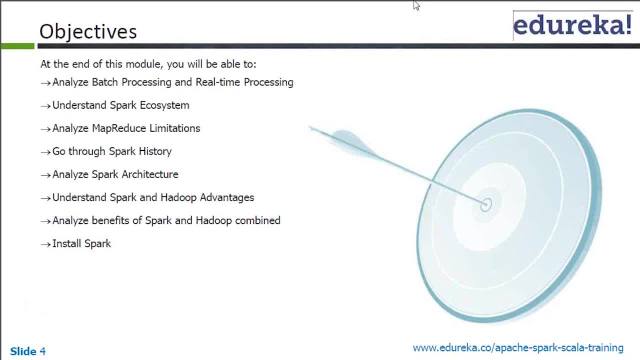 The MapReduce limitations, okay, But then it would lead us towards the SPARC history Again. SPARC history is something which I don't, Where I don't like to spend more than one specific slide, But the idea would be how SPARC is really different from the other. you know. 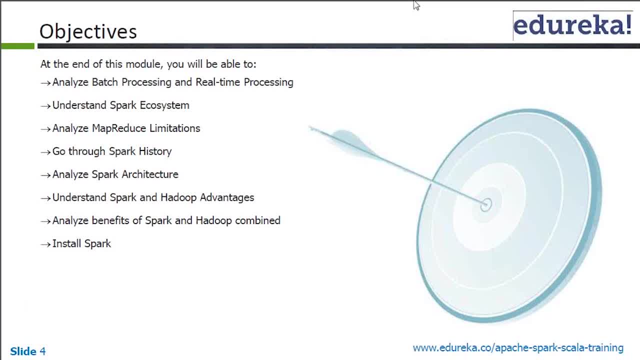 other specialized big data solutions. So we will come to that part And then SPARC architecture. I would say that probably, if I would be able to cover up the history part today, it would be good And start a fresh and SPARC architecture. 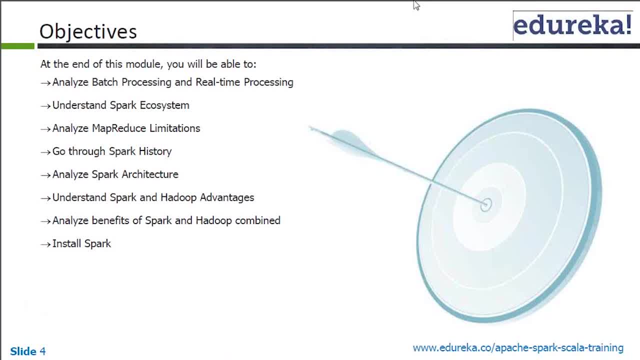 Because I don't want architecture thing to go at the time when you are, you know, when our information registers are full right, So I don't really want to go there But still. So the objective would be SPARC architecture And then one of the much important buzzwords which are kind of today, you know. 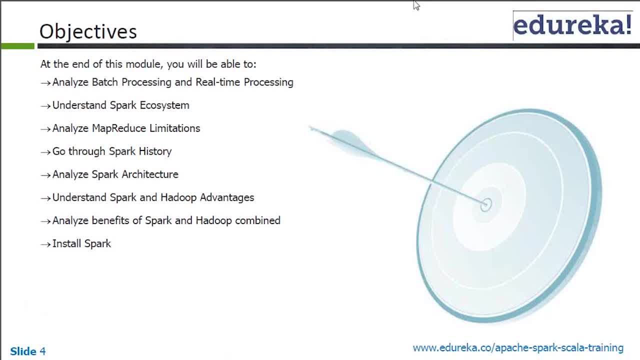 doing the rounds. it's about SPARC and Hadoop. So people you know, talk a lot about SPARC, Hadoop and all, But you will see that, what it takes, what does it mean when you say SPARC plus Hadoop? 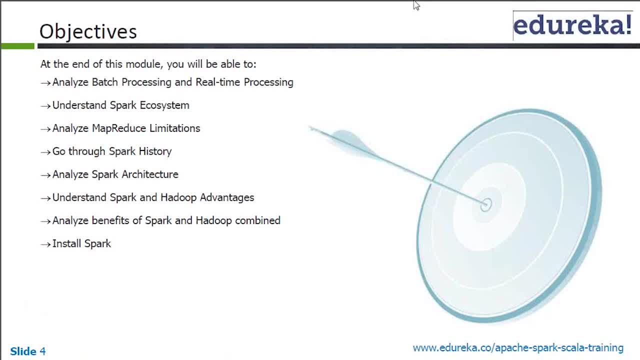 It has got different meanings, okay, depending upon how you are going to use it. So we'll discuss those aspects And then, rather than install SPARC basically here, I say that you know. please refer to the installation document which we have shown. 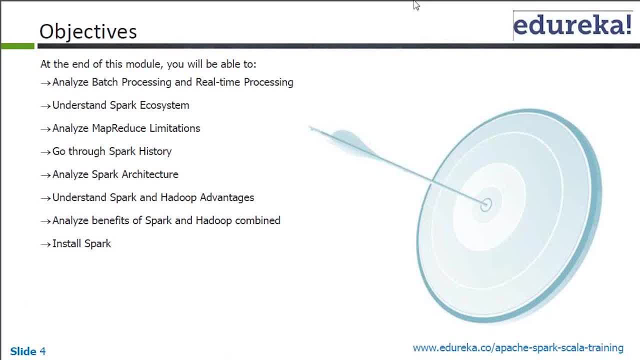 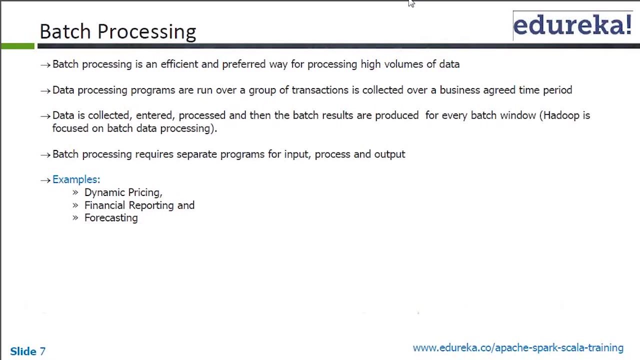 But again, instead of this, install SPARC. basically, I would be spending some time on SBT. part of it Is that. I hope that should be quite clear with everybody, right? See, you are having a huge amount of data. You want to process them using one of the big data systems, altogether okay. 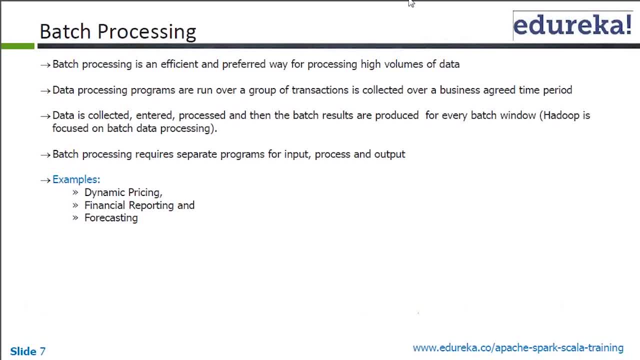 Now point is, you must have heard about batch processing and real-time processing itself, right? So what exactly are the best examples for it? So, guys, batch processing, when you typically talk about it, I would okay. let me just give you one simple example. altogether, 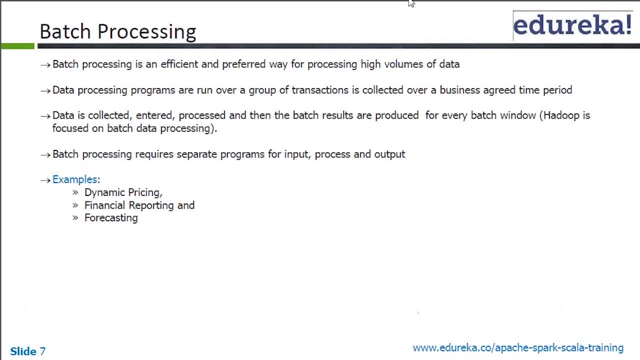 Let's say you know you are having your retail industry. I'll give you the example of retail industry. You are having your stock ledgers, your general ledgers. They are the typical ledgers which are there in any market, Any of the retail industry. I mean retail, whatever major you will talk about. 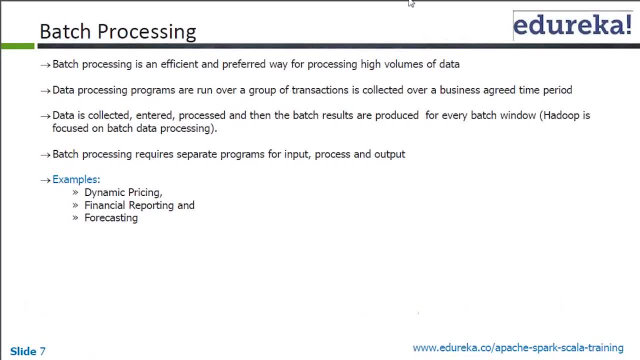 even in the. they are common concepts in the banking industry as well, But let's say in the terms of: you know this specific retail thing Now. so what exactly happens on the stock ledger side? and all Those stock ledgers are something which typically have the inventory information, altogether right. 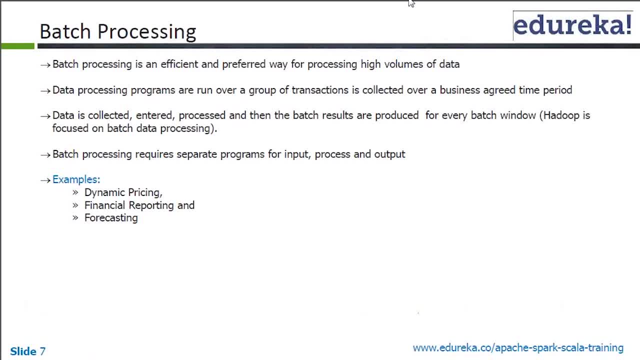 With the store, this particular division, this particular you know item, this many number of you know overall quantities available and the kind of price and et cetera, et cetera. And this stock ledger is something which keeps getting updated every day, right, 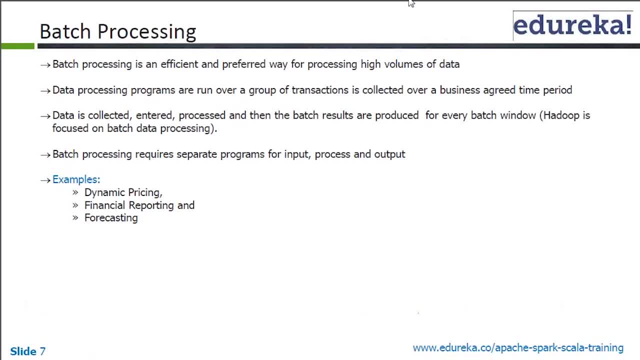 Sales have happened, theft, you know, and all that right, So they just keep getting updated And then at the end of the business day you have to, kind of you know, close your business and before you start next day's business, 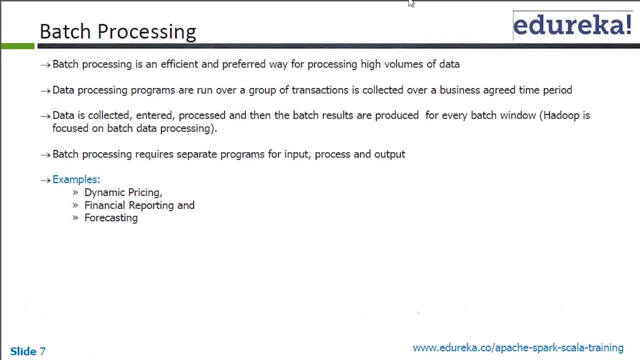 all of this has to be consolidated and your kind of. you know targets, whatever there are. there are any kind of forecasts. you know financial reporting, basically So, if there are any kind of forecasts or if there are any kinds of targets which you have to set. 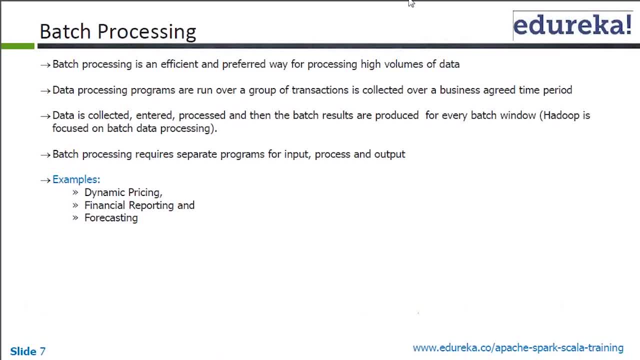 they have to be updated before the next business day starts. And what is the best way to do that? The best way to do that is take all of the transactions which have happened in a day. You don't really need to. you don't really need to do all of this again and again in a day, right? 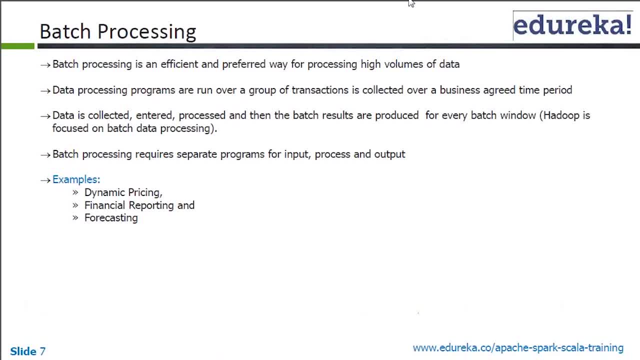 You have to do it once in a day before the you know next business day starts, And so, basically, when the today's business day ends and before the next business day starts, right In between, you have to do this process once. 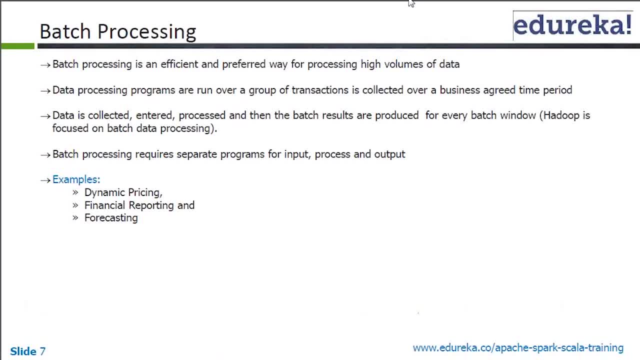 Are you all getting the point, Guys? are you all getting this point? So if you talk about this this typically, that the processing which you would do in this case is once in a day, it's kind of a batch processing altogether right. 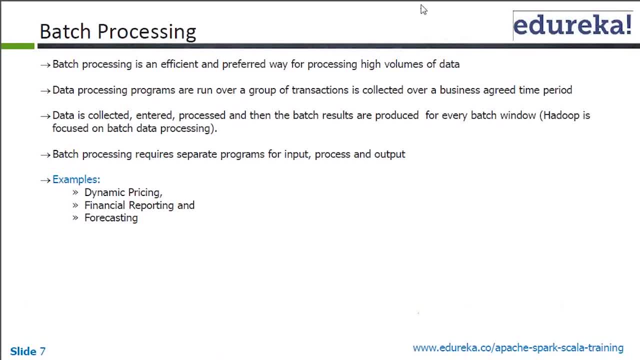 Now, when you talk about guys, are you all hearing me? I mean, I'm not really sure whether I'm getting your response or not. Okay, Great, Yeah, Thanks. So you know your response actually tells me whether it is clear or not. 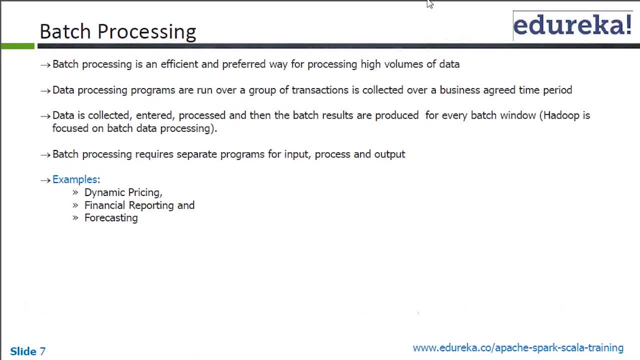 Or, if there is any question, it can be Right Now. so batch processing is going to be your- you know- preferred way. So when you talk about big data applications and all, it's the preferred way of processing huge amount of data. 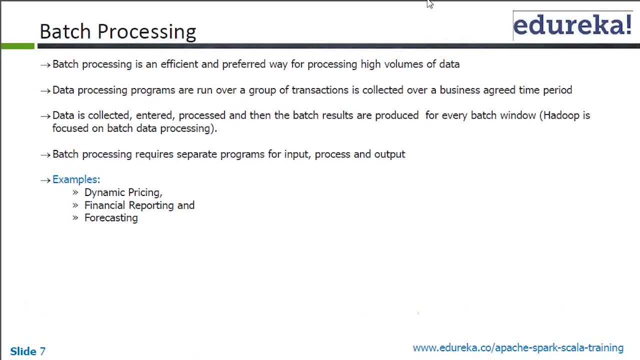 And typically what happens is you group a lot of transaction over a defined period, right? Basically, it's going to be the frequency of your batch job: Once in a day, weekly or whatever. Twice in a day kind of a thing. 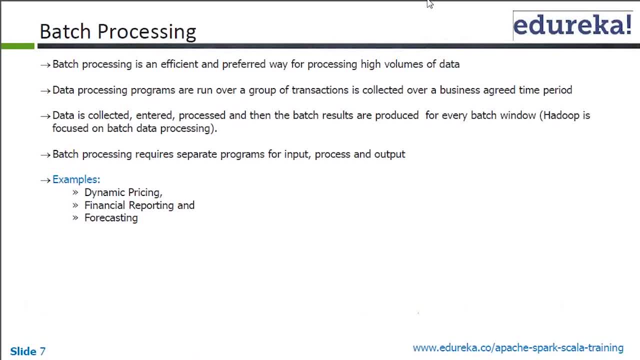 Right, So you'll be collecting that huge amount of data, processing it in a given batch window, Right? So batch window means in a, you know whatever The time period in which the batch runs, So that is typically called a batch window. 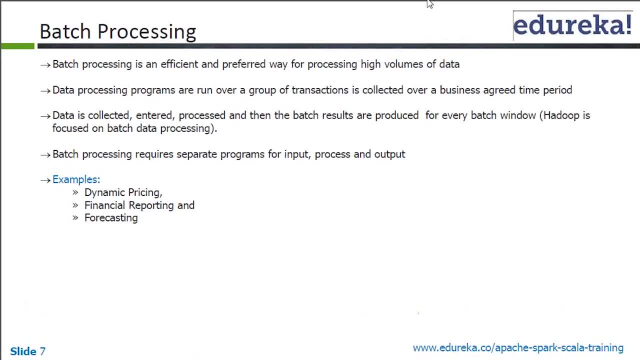 And Hadoop is typically used for the batch processing. Nothing new Examples, I think, like financial reporting, forecasting, dynamic pricing- Though dynamic pricing in some cases it has become kind of real time as well. But I'll probably come to that when I talk about the real time processing. 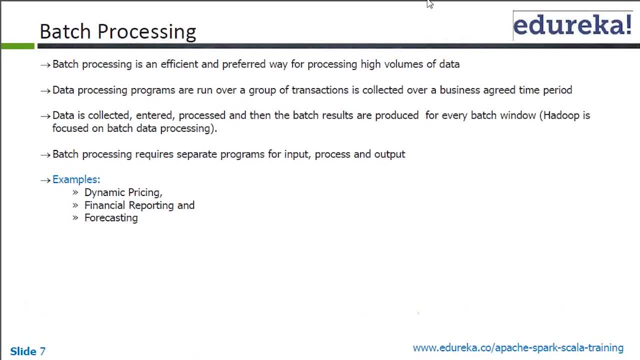 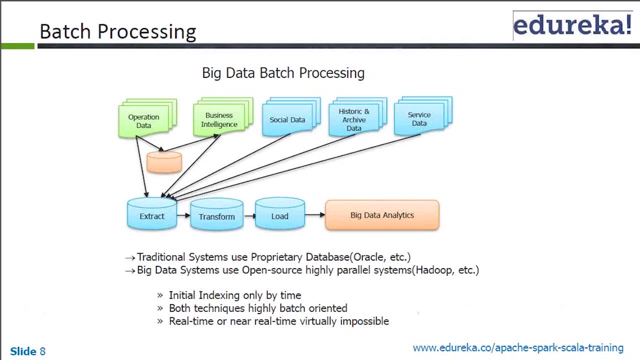 Right. So they are typically called the batch processing kind of systems And we are quite well versed with them And we are using Hadoop also for them since quite a long time. Not a problem at all Right Now, if you just move, it's a very generalized kind of way. 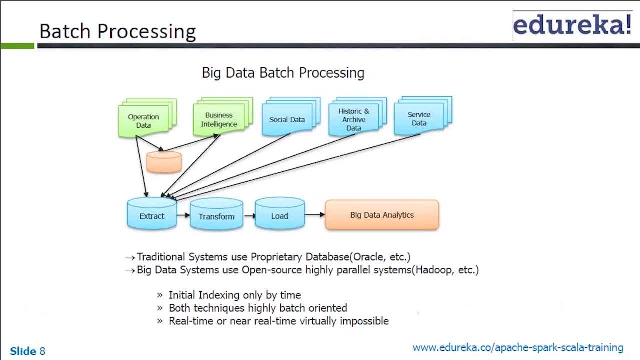 So you might be having multiple data. You know sources all together: Social data, BI data, operational data, et cetera, et cetera, et cetera. You must be putting them into. you know your data lake. 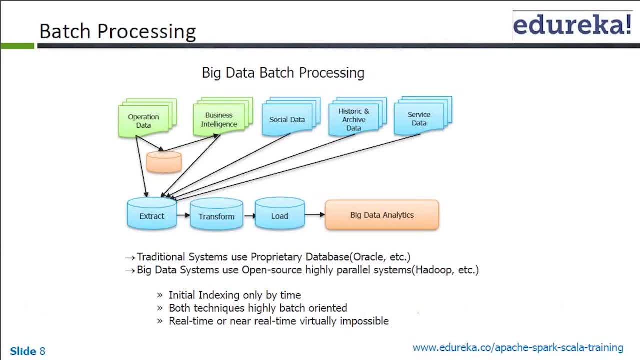 If I don't call it as data lake, let's say in a very simple manner: You're just, you know, Hadoop of processes which will be applied, And then you will be doing whatever analytical functions you want to do. Right? 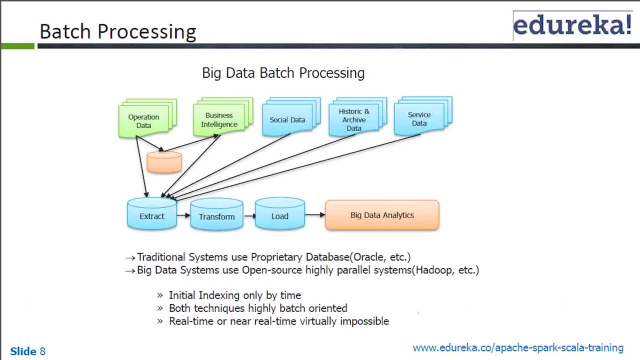 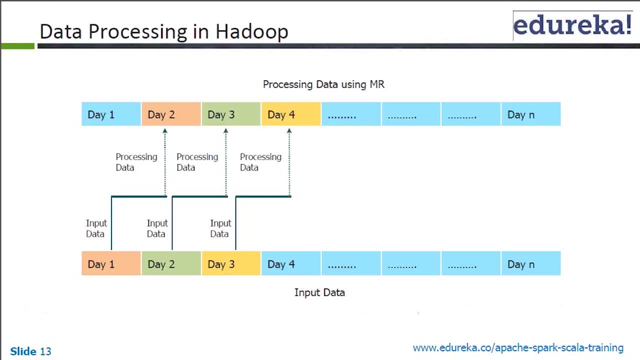 So good thing, But So what really happens in this case is something like it. Just a second, guys. I don't want to cover real time processing right now. Okay, I will come back to this slide, guys. I will come back to the slides which I just skipped. 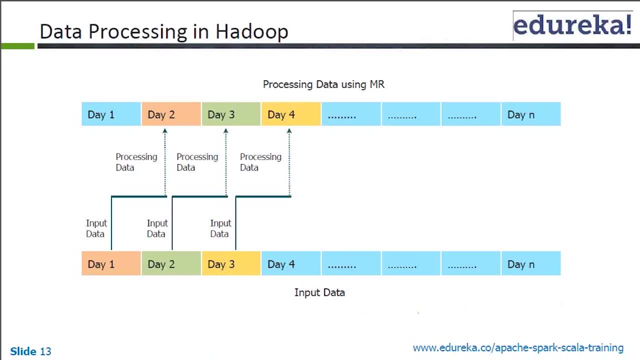 Okay, So what really happens in this case? In this case, let's say, if you look at about the data, this is your input data, Right, This is your input data kind of you know timeline And this is your processing timeline. 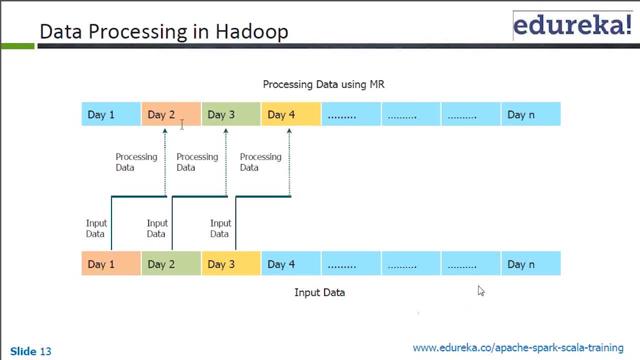 So, assuming that it's a daily process, So whatever is the input data of day one that is going to be processed in day two And basically it's going to be one day delay altogether, Right? So all the time if I'm looking at the data, if I'm looking at some of the report, right? 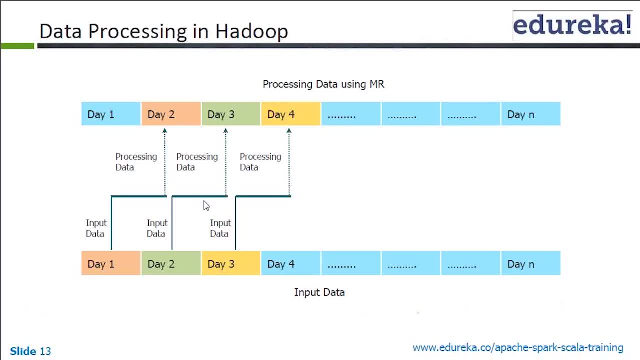 now I am quite sure that things have changed Right. So the data which I'm looking right now, This is: whatever is the actual, whatever should be the actual view. it's kind of a stale view, Right. I'm not getting a fresh view all the time or hot view all the time. 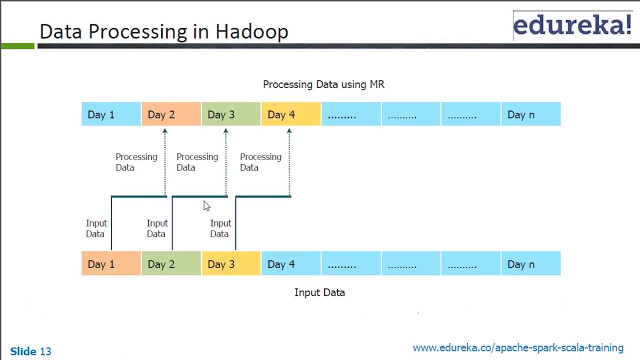 Right, It is just that I'm getting some sort of pre-processed data to a certain frequency, which might be a day older, which might be some two, three hours older, kind of thing, Right, Depending upon what is the frequency and all. 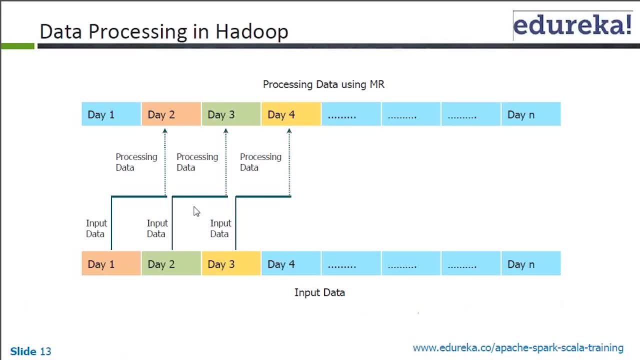 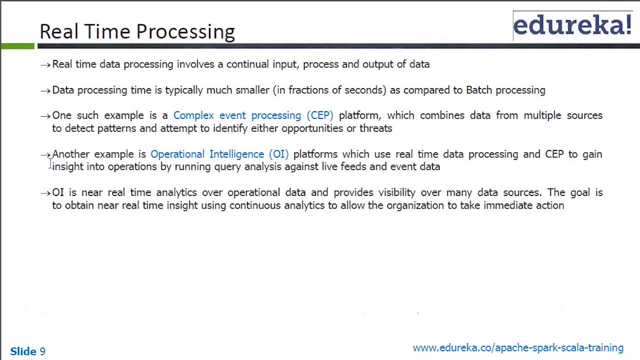 Right. So this is quite good for batch processing, But now let us take a step back. Okay, Let us take a step back and talk about real time processing. Now, when you talk about real time processing, first of all, before I read any of these points, 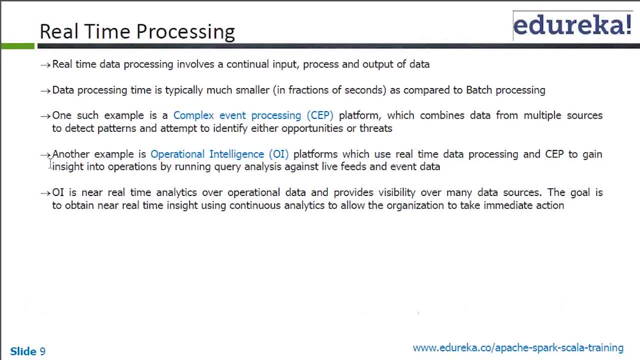 let me explain that real time processing is nothing, but it's a myth. There is nothing called real time processing in big data world. Okay, There is absolutely nothing called real time processing. At max it is near real time processing. Okay, So it seems like somebody is saying something. 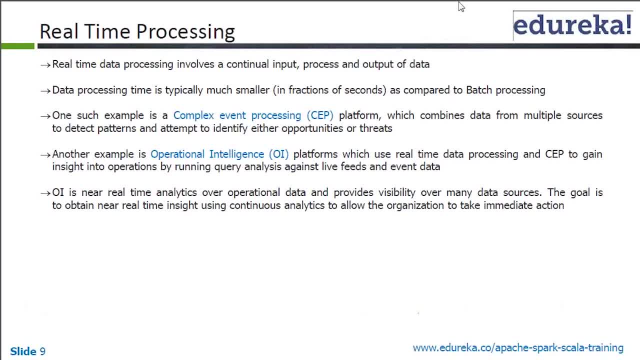 Streaming, Again Satish. these are different ways. I will come to that. I will come to that Streaming is big, Okay, But point is, be it streaming, be it Hadoop streaming, be it the streaming way or be it. 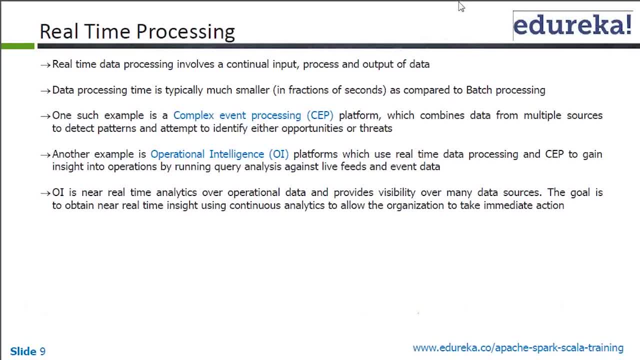 the Spark streaming. all of them are the example, or the best examples, for near real time processing. They are not at all the examples of real time. Let me tell you one of the examples which I have implemented in one of the banks altogether. But before that let me just tell a bit more about real time processing. 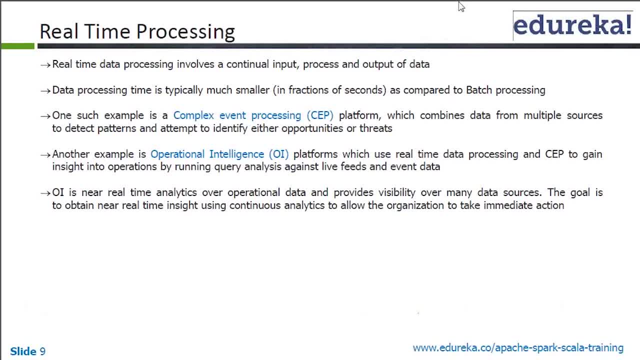 So real time processing itself is all about your data processing. Data processing is going to continue. Okay, It's not like a, you know it's going to work on a continual input altogether and it's going to work on those small chunks of the data and it will keep on outputting the data. 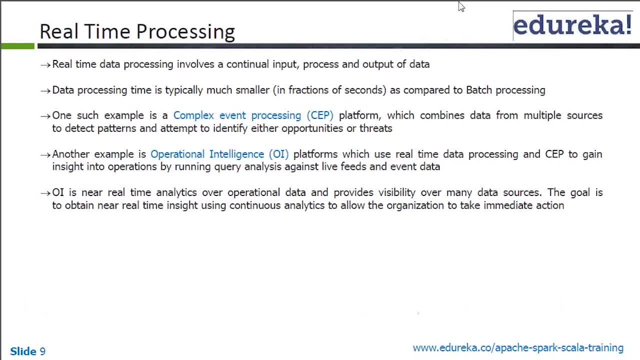 again and again. So the idea here is: in the batch processing, your applications were running again and again in the larger interval, Whereas here, Here, Here, The interval itself is going to be very small. Okay, So your program is going to execute again and again. 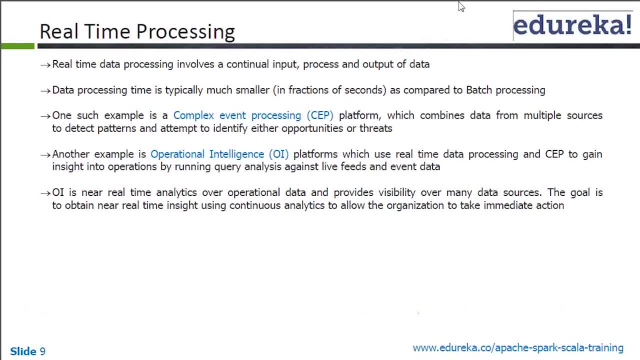 But in the delta time, whatever is the extra amount which came, you immediately process it and show the output. Now, this is the basic difference. here You talk about real time processing. When you talk about real time processing here most of the applications, I mean you can. 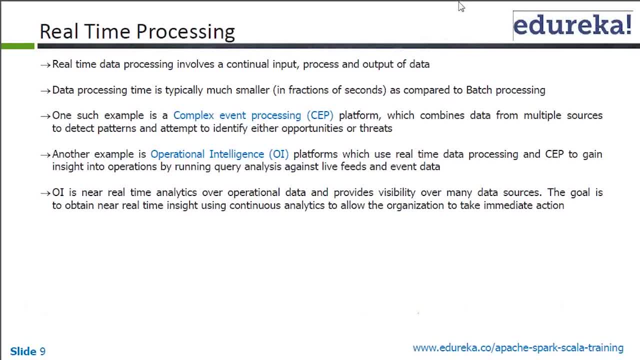 modify them. But, at the very essence, Most of these real time- so-called real time- applications are for the sliding window type of operations. Okay, So most of these are suitable for the sliding window operations altogether. So, for example, trending topics in last one hour. 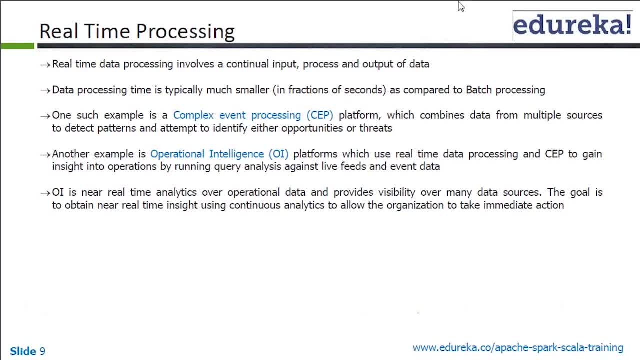 Right Or trending topics in whatever last n number of minutes altogether. This is a sliding window kind of operation Right Wherein- right now probably, I'm just giving an example. Okay, So probably up to yesterday, yesterday night, Modi's, Mr Narendra Modi's US visit was a. 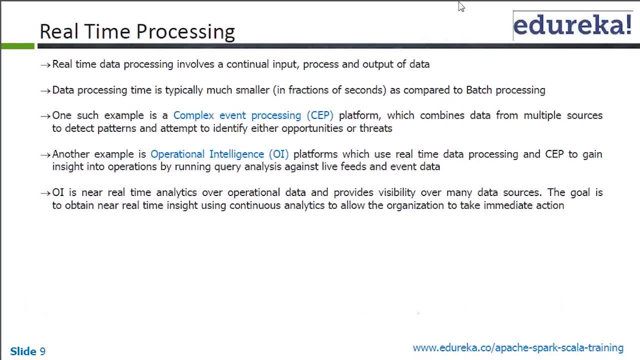 trending topic in Facebook, in most of the social media Right. I'm just giving one example. But from 12 o'clock up to, let's say, morning 4 o'clock, there was an incident in India. Some accident happened or I don't know. 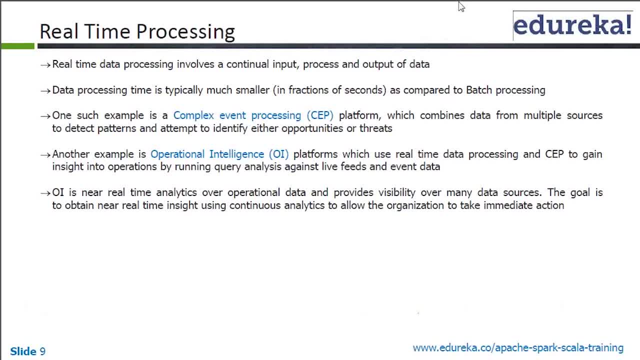 Some other thing, Right, Some Dasharha celebrations and other things, Right. So they have just started here itself, So this has become a trending topic altogether, Right? So if you look at it, what happened before that was not really a problem. 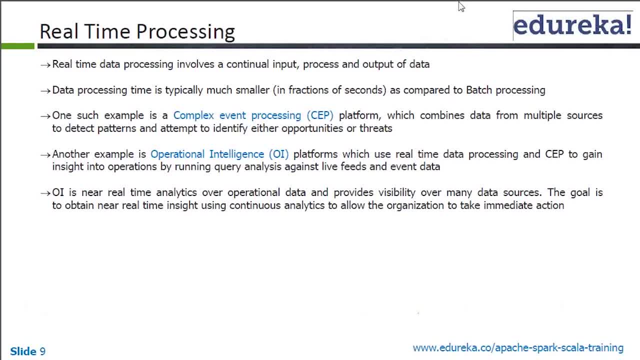 So if you look at it from the batch processing perspective, if you had to implement these kind of trending topic kind of you know algorithms altogether in a batch processing way, probably you might not be getting the latest picture, But if you have to do these sliding window operations typically you would like to go. 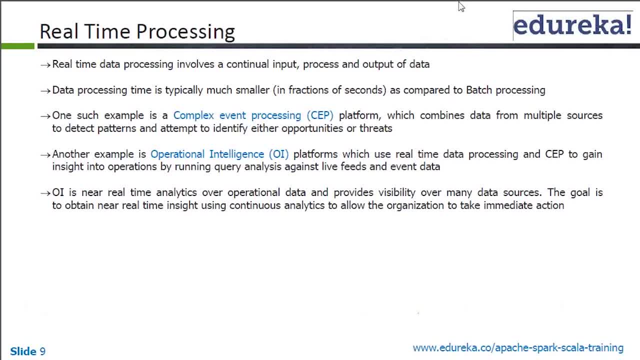 for something called near real-time processing kind of system altogether. or let's say there is an event number of tweets which come on the top of it. this is the real-time processing kind of examples. So here the data processing is typically much smaller. it's going to be usually in 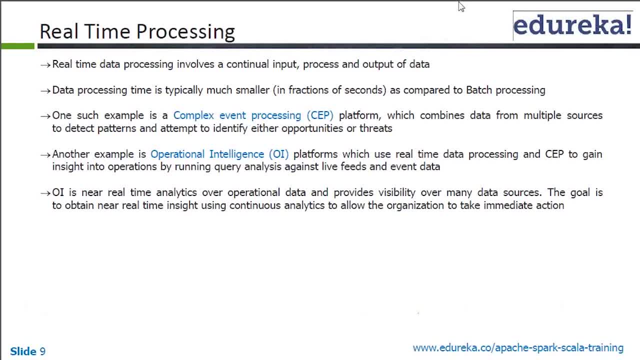 the fractions of seconds and as compared to the batch processing, because there the batch window will be at the fastest- would be several minutes. right, The typical use case of real-time- or assume that I am talking about near real-time, so about the real-time systems- would be CEP platforms, altogether complex event processing. 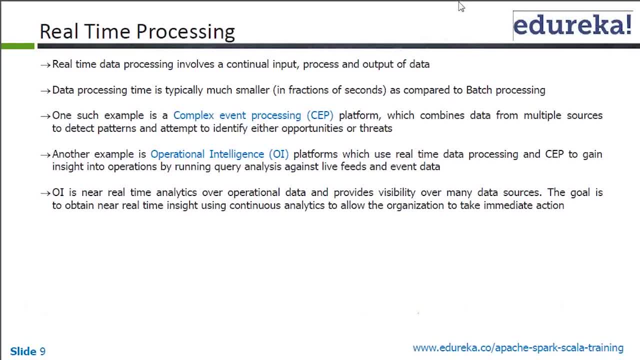 kind of platforms. So what is the best example of it? So the best example of it is, though we have not implemented any big data solution for that. It's kind of a cousin of STORM in which I have implemented. it's called ESPER, okay. 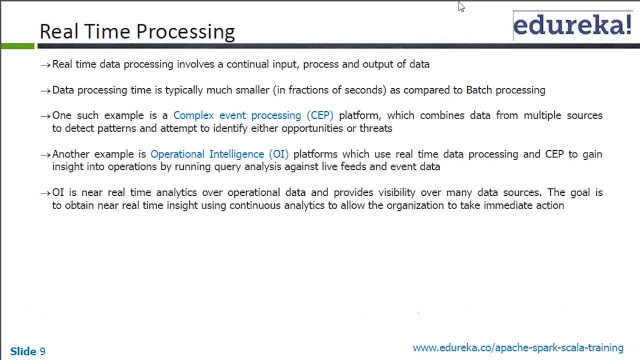 So what happens is: let's say you are doing a transaction- okay, credit card transaction, simple and online. let's say you are purchasing something, you provide your credentials, whatever X, Y, Z, and everything is well. you are. you know. you are well within your limits. 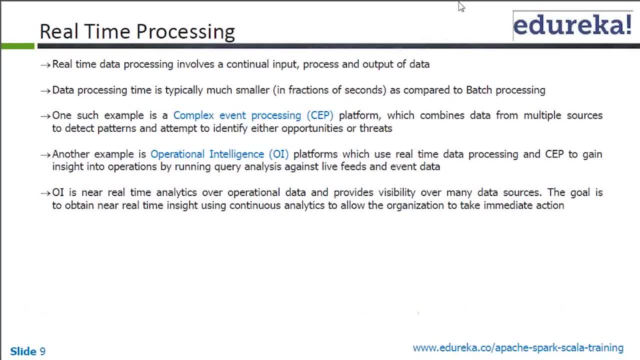 you are buying, Buying something, your credentials and everything, whatever you have provided, is good and the transaction happens successfully, okay. So, for example, right now you have done a transaction very good, everything is, everything goes well in the banking world, altogether good. 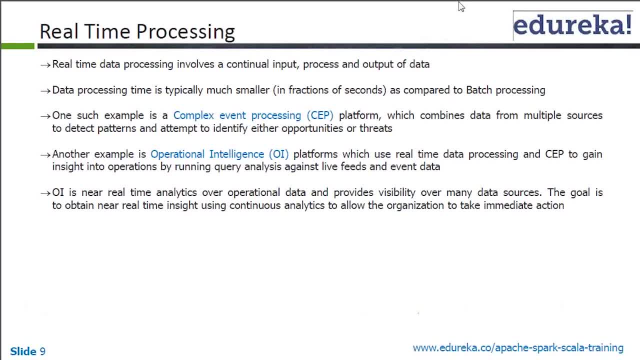 Now, let's say, one hour later, one more transaction happens on your credit card. okay, Credentials, and everything is good. everything is good, okay, Okay. And then the transaction, next transaction, whatever is happening, again falls within the credit limit. no problems at all, everything is good okay. 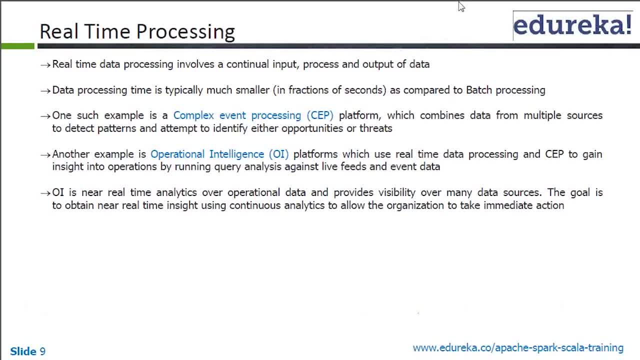 But there is one thing that the first transaction, the geographical data, which, when you, you know you agree that, okay, I am ready to share my location, right, and when you are sharing your location, it found that the first transaction originated in Delhi. okay, but the second 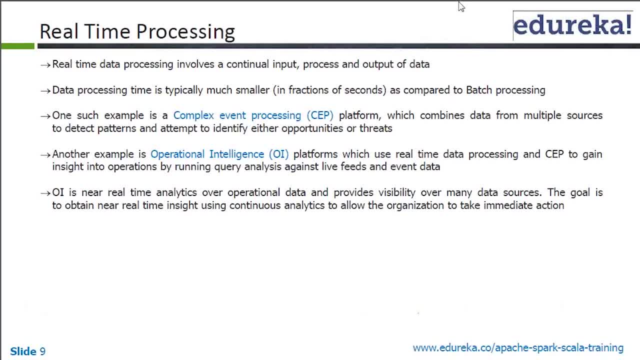 transaction one hour later is happening somewhere in Mumbai. right Now, it is physically impossible for a person to be there at two different places at the same time, right, guys? I hope you are understanding the point, right? So now, if this thing has to be detected, right? so, even if everything is good, but 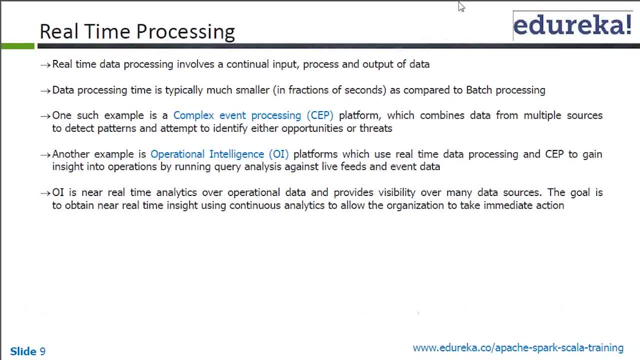 if the geographical data shows something. now there must be a program. I am just giving you an example, I am just giving you a hint. I mean we have implemented it in that way, okay, So there must be a program which will continuously run on a stream of data which is coming again. 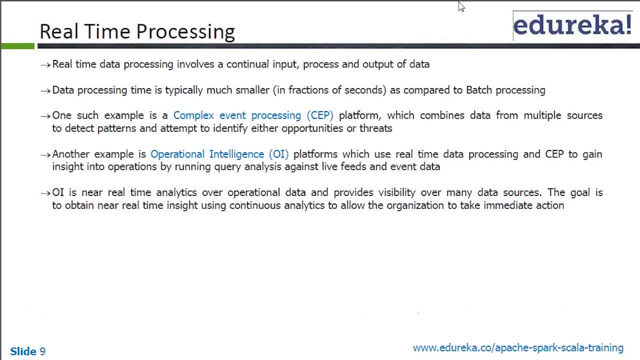 and again, right. So, and this program might be somewhere before your request is sent to the payment gateway, right? If that program boolean returns, yes, then send it to the payment gateway. If that program boolean output is false, then either reject it or send it to something called. 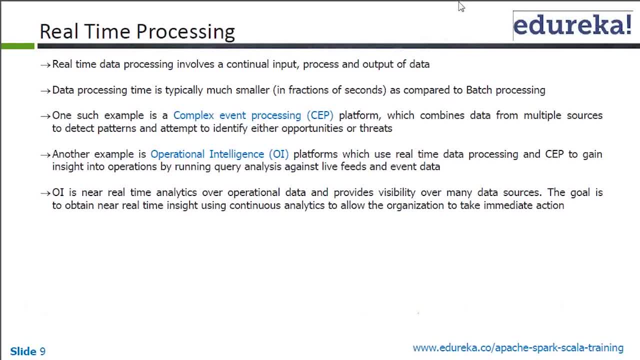 referral right. So referral means what would happen in that case? as soon as the transaction would happen, you will get a call on your registered number, okay, saying that, sir or ma'am, we are seeing this particular transaction happening right now on your card with this thing. 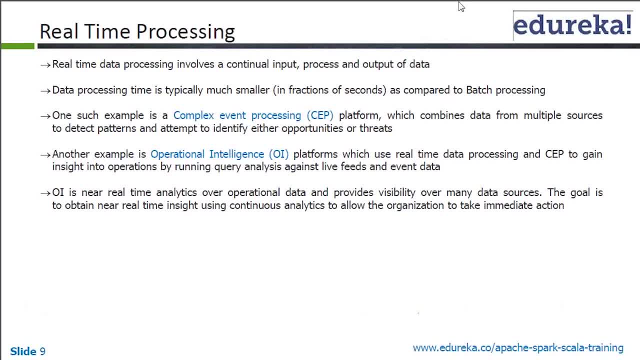 Is this you who is doing the transaction? Has it happened with any of you? Because the bank for which I have implemented is a renowned bank. That would give you the idea as well. So, anyway, for the processes, they are now planning to move it on a larger scale. 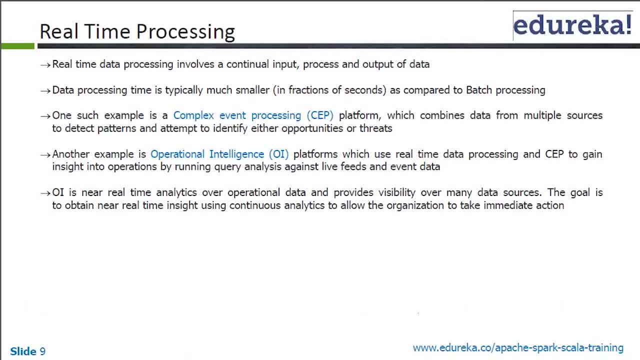 It was a POC, So not many of you might have got it, but yes, it was implemented for some certain reasons, and then I think it is in the process of Bank of America as well. Might be, might be, might be, Satish right. 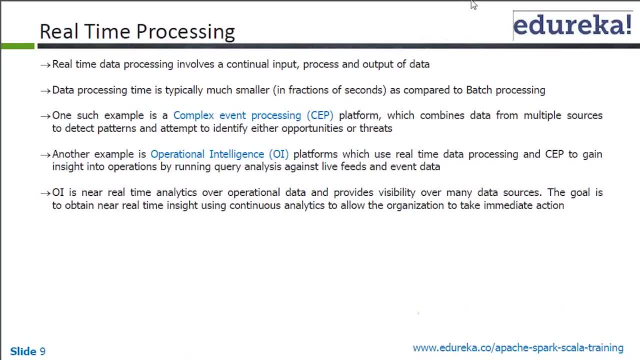 So there are several that I'm just sharing my experience, right, Okay, now let me just quickly come back. So those kind of systems are called complex event processing platforms. Now look at it: This, what, what are? the focus point is not really the implementation. 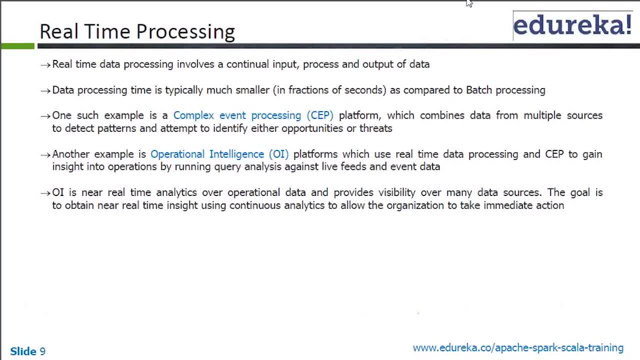 The focus point is: look at the way you are going to process your transactions. You are interested only in present. You are interested in seeing that. okay, what is this transaction which is coming at and that's it. They don't really care about what happened in past, what will happen in future, right? 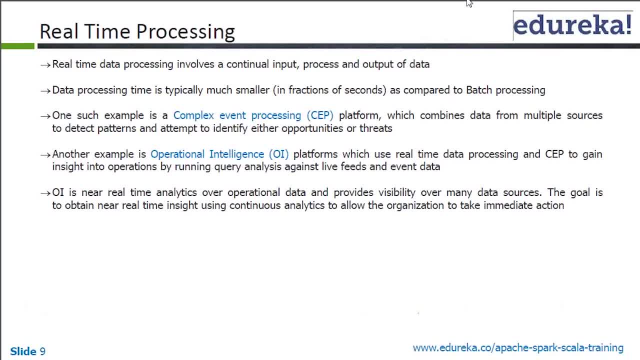 There was one program which was written and which was just seeing that, okay, whenever a transaction comes, just look at it, the last transaction and the time, and if whatever, right. And then just see that if that is good, good, Otherwise, you know, just send the request for the referral. altogether right. 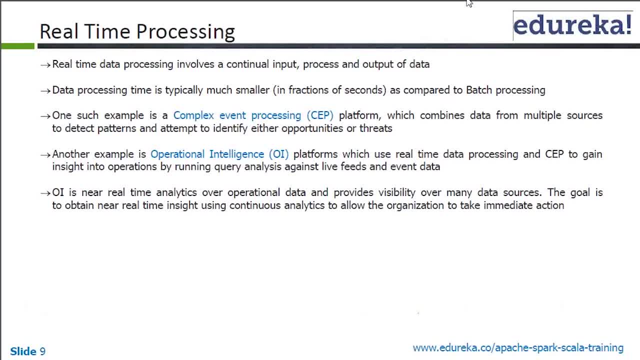 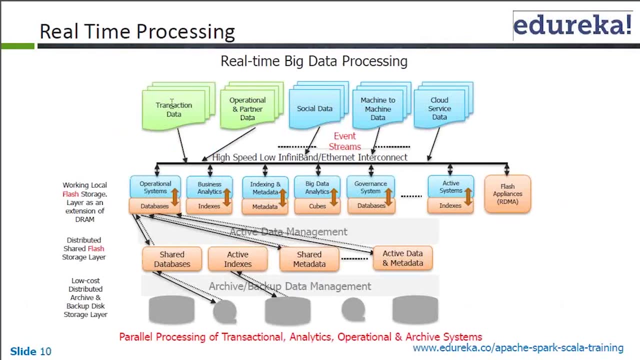 They don't really care about past or they don't really care about the future, That is. that is the basic difference altogether of the, you know, real time processing systems altogether, right, So I have, though I have not covered this part, okay, I am not trying to confuse you here. 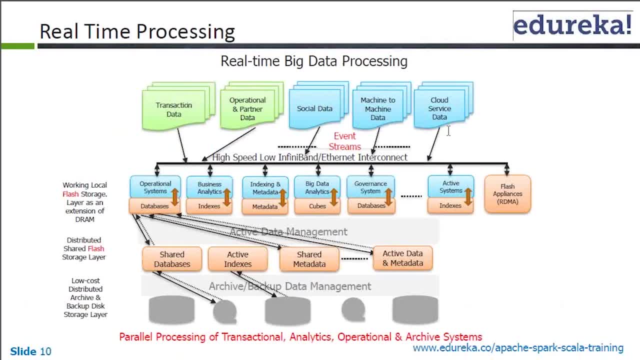 It is all about. you will be having multiple data platforms. then there would be a shared metadata, kind of a layer. These are typical ways. okay, these are typical ways in which you know you create your real time systems And then your small, small real time systems would just be: you know you create your real 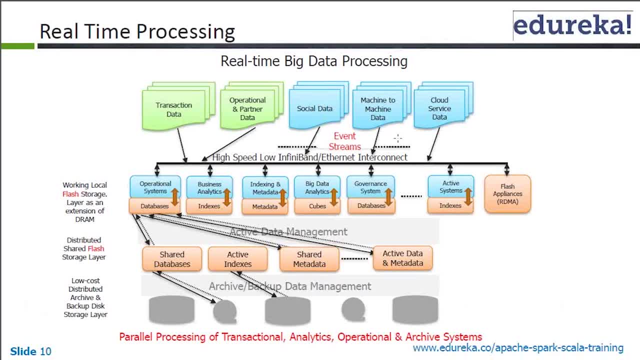 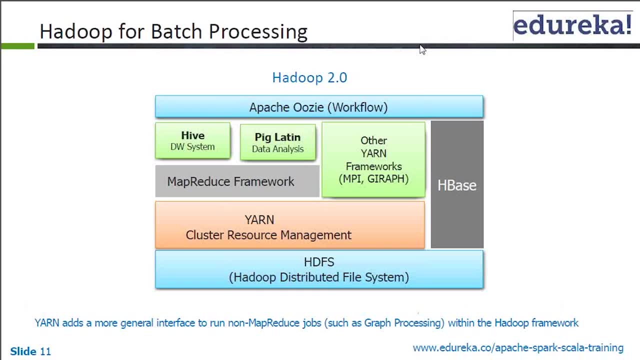 time systems. Okay, So they would be working on this data, shared metadata, altogether. they would be working and then they would be generating some sort of notifications. okay, So most of the times, your real time systems, or so-called real time systems, are used for. 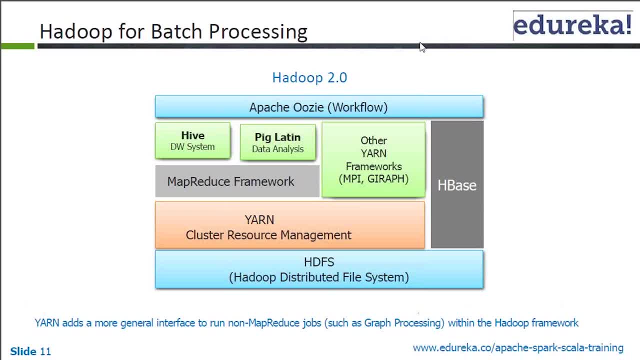 the event processing or for the event notification and not really any processing. So any processing when you talk about the processing, the processing of calling you, confirming the things and all happened by some other bank Bank enterprise system- right, Your real time. enterprises, your real time. you know, big data system didn't do anything. 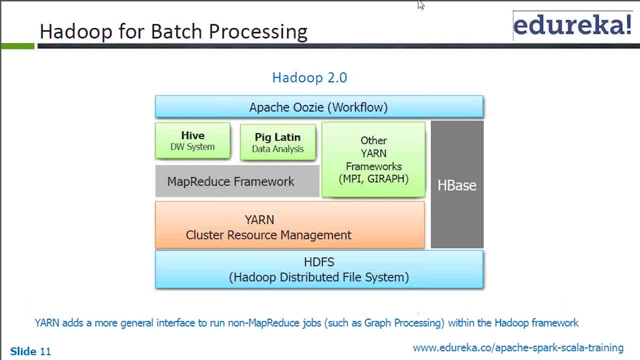 Are you getting my point? Your real time big data application didn't do anything other than passing the request to the right person, passing the request to the right application altogether, and that's it. Its scope is over. Is that clear to everybody? The basic difference. 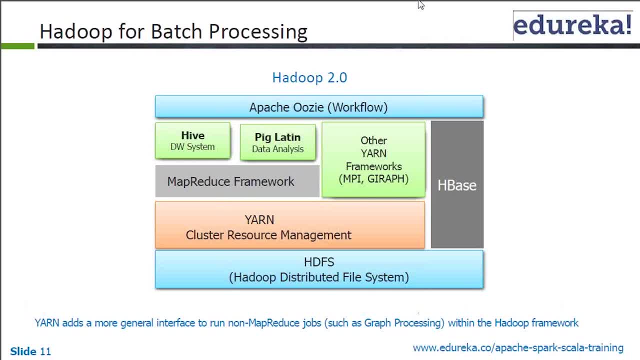 The way you should go for your process. Okay, There are some problems, right, And also it's called real time also because there is no point of saying that this was a fraud transaction when the transaction has happened. right, All of the referral has to happen before your request goes to the payment gateway, right? 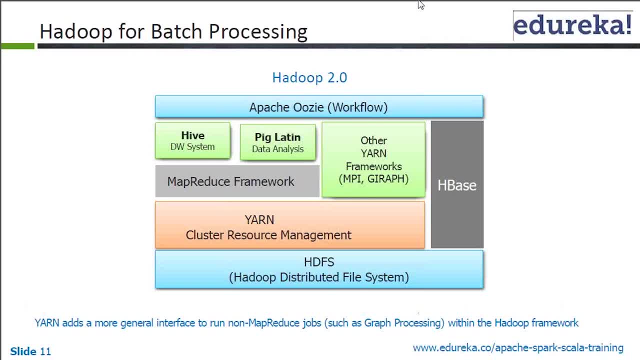 All of this. So that's why people call it as a real time system, right? So these are some of the things where you have to think So when you are going to apply Spark, right? Spark in some cases can be used for real time. 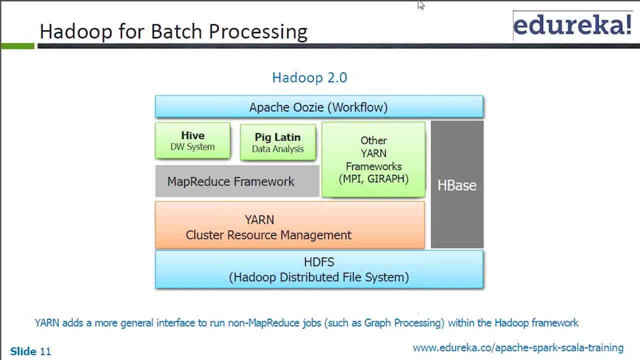 processing, but most of the places its typical use case is going to be very fast biased processing. Okay, So I would give you another best example for which we are kind of so. there are two POCs: One is in the- we are about to productionalize it, and another one is in the POC stage, wherein 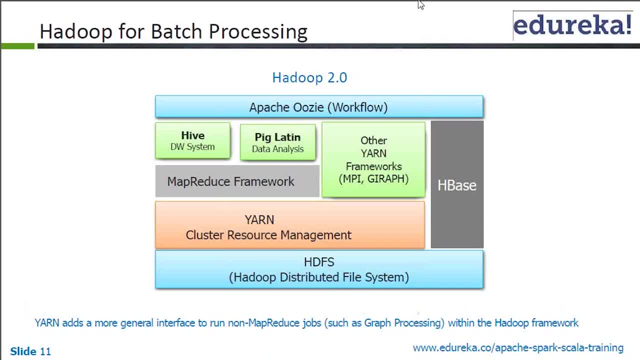 we are just trying to enhance it a bit more. So one is called dynamic pricing. I am sure I'm not going to spend much time on the dynamic pricing It's all about. you know that depending upon the demand, your inventory, you know prices. 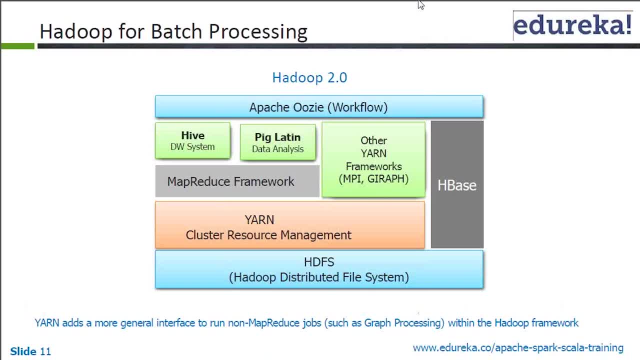 have to be dynamic. They have to change very, very fast. Okay, So that was the place wherein we have applied Spark processes and they have kind of you know. So now, basically, this retailer- I can't name it right now, but this retailer has now. 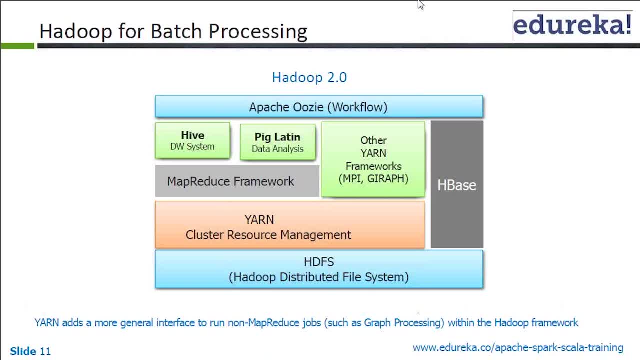 applied this dynamic pricing module and it runs kind of every half an hour. Earlier it used to run once in a day and then when it went to Hadoop it was running twice in a day. okay, But now with that it is running every half an hour and they are able to get much better. 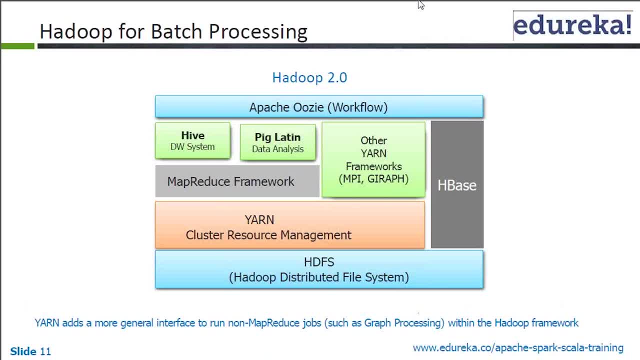 responses or much better margins altogether. Okay, So, So this is just one example. I'm just giving you one example about the suitability. See more than the language itself or more than the framework itself, these kind of questions will come to you when you will be implementing these. 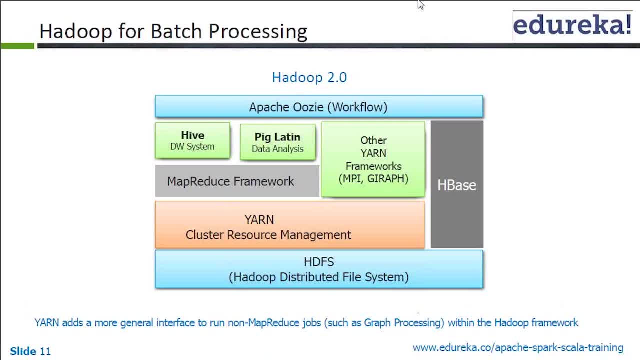 Should I implement or is this the best fit right? So just keep these things in your mind And that's why this entire discussion- one-time discussion- is happening with you. okay, So Hadoop for batch processing. I'm not spending much time on it. 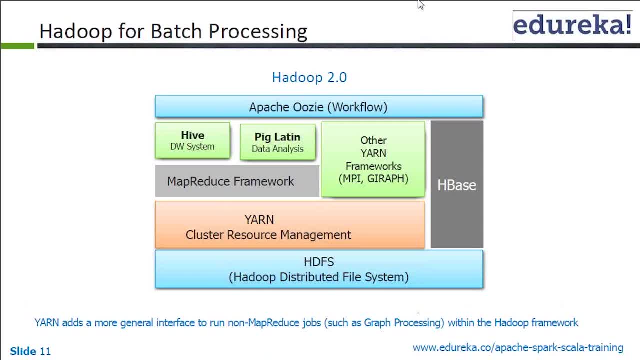 It's about. So the overall purpose of keeping it here. only It is for those people who are not aware of Hadoop right, There are several here. So HDFS it's the storage layer, and we have covered only Hadoop 2.0.. 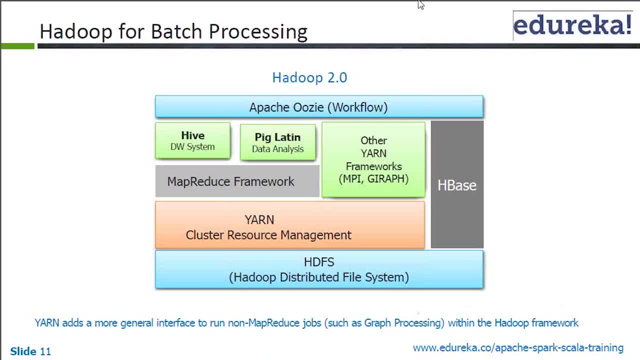 We are not showing Hadoop 1.0 because that's the way forward, right? YARN, that's your cluster resource management. and then you have MapReduce framework, on the top of which you know Peg and Hive can run, And then you have other YARN frameworks, right, which are like your Giraffe Spark, right? 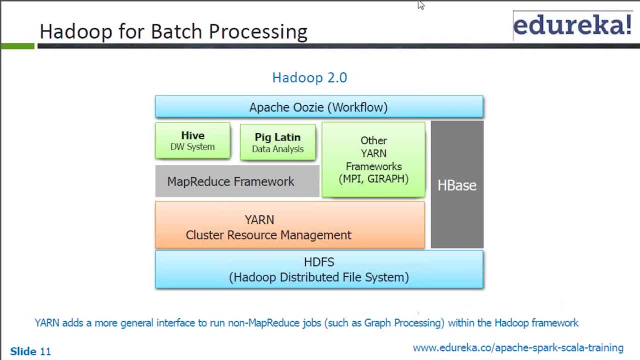 And there are several other frameworks, Okay, Okay, And there are several others as well: Pregel, Dremel, etc. which can run on the top of it. And then you have HBase, which is which kind of, you know, directly interacts with HDFS. 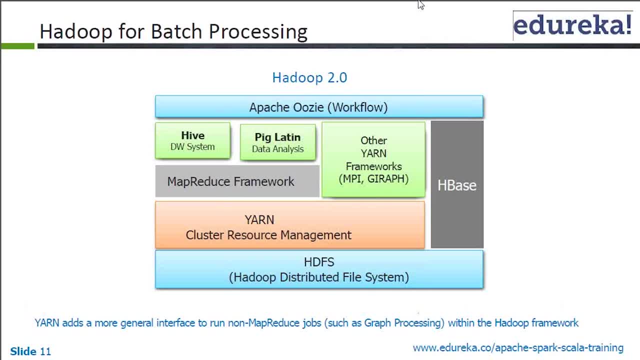 without YARN, And this remains unchanged till now as well. right, So this is something wherein your typical, you know, Hadoop ecosystem is, and on the top of it you are seeing Uzi. It's all about your workflow, Shadyware. 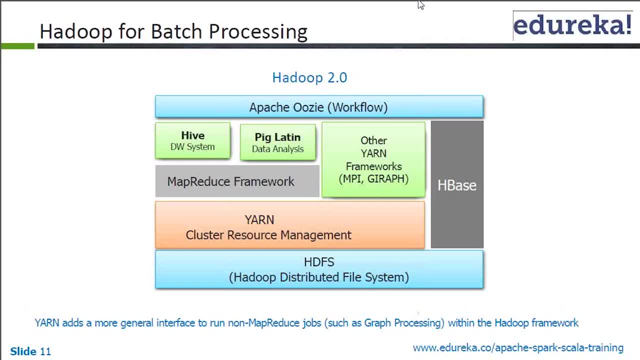 So you know, In a job you might do some sort of scoop and then do some sort of pig processing and probably, you know, persisting some data into HBase and then doing some kind of fetching it right into, let's say, a UI. 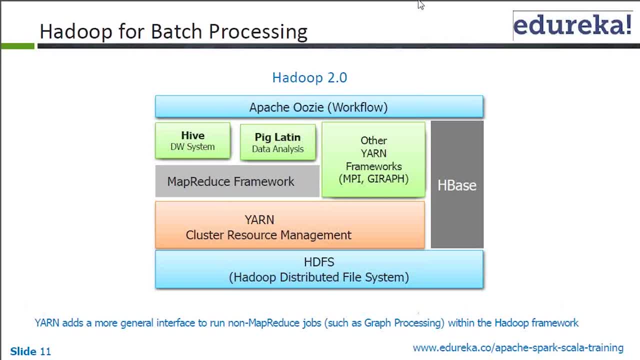 You want to do these things in one by one order, and if there is any failure, you want some sort of decision points, etc. Those are some of the things which you can do in workflow Shadyware, which is Uzi right. 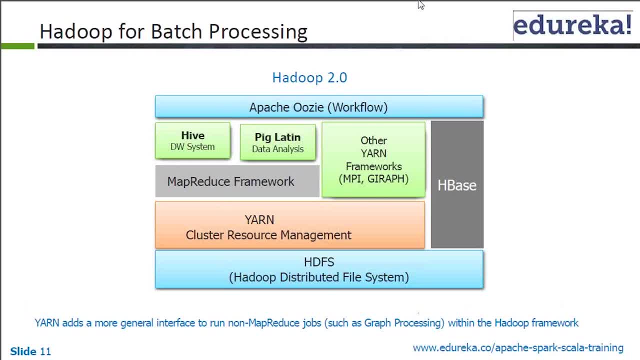 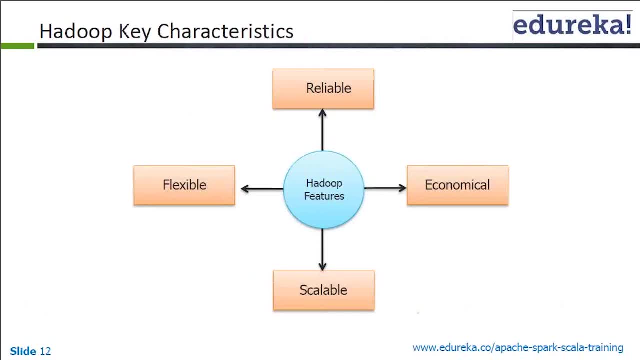 So I'm not spending much time into it. I hope everybody understands it. Right, Great Now. so again, some of the Hadoop key characteristics and all which are quite clear, and those people from Hadoop classes must be able to recognize them as well. right, 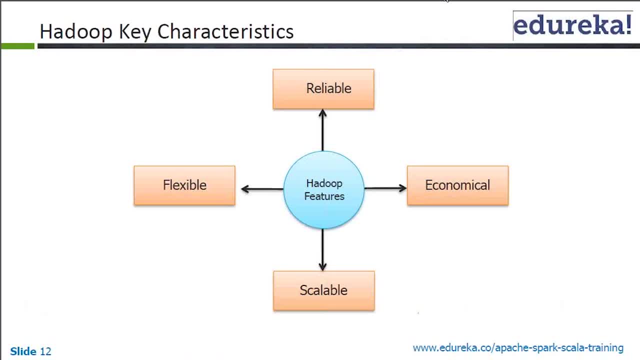 So quickly. it is about scalability. So again, since it's a Hadoop cluster of commodity hardware we are talking about. scalability is something which you already get Economical, of course, because you're again, you're talking about the commodity hardware. 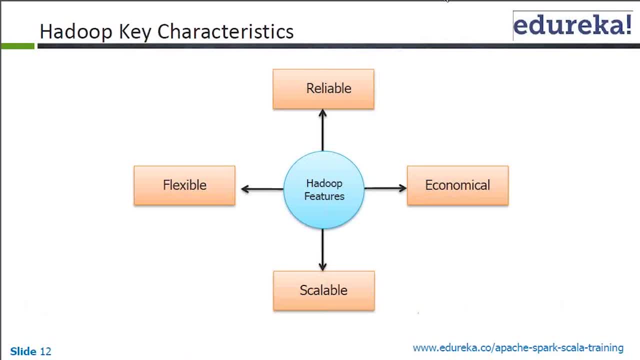 which is, of course, going to be more economical as compared to industry grade. you know those big servers and all right and reliability side, so which is built in within Hadoop, So it's really good for your, you know, batch processing itself. 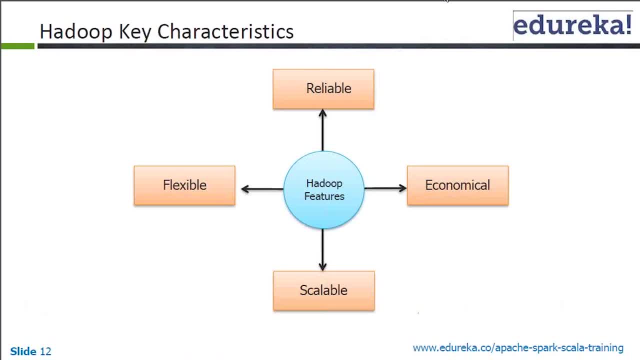 If there are any failures, auto scheduling it, speculative execution and, you know, auto replication altogether. So some of those things. And when it comes to flexible, it's quite flexible, and so when we talk about it, you can either deal with the structured data, unstructured data, semi-structured data, etc. 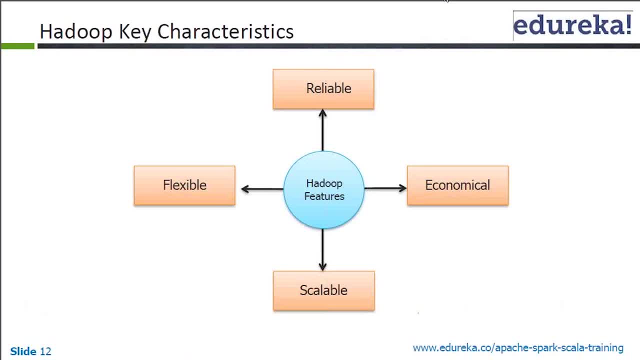 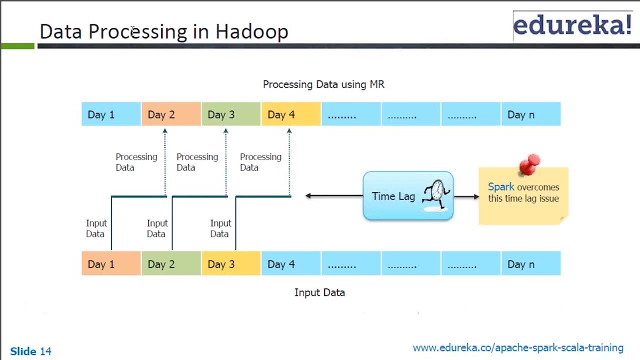 So these are the typical Hadoop features. By the way, there is a reason of spending even those you know. we have chosen, very, you know, picked and chosen very specific slides for it. okay, There is a reason behind it. 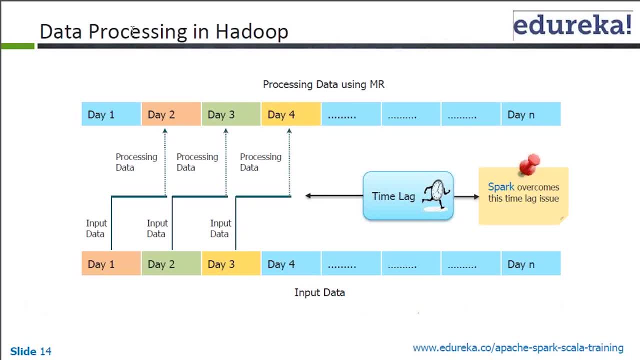 You will be very, very clear about it when we will come to Spark plus Hadoop. Okay, So that's the direction in which we'll move. I hope data processing in Hadoop is quite clear to everybody, right? Basically, I just wanted to show you this is a batch processing system. 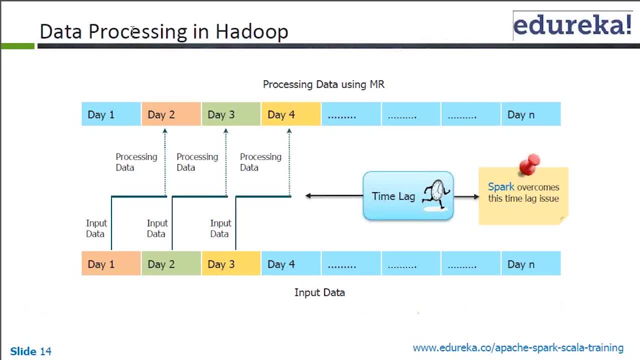 It is all good, but the problem for you is that one day delay kind of a thing, right. So it typically leads to the time lag, and this is where, basically, Spark comes in between. Spark overcomes This time lag, This time lag issue. 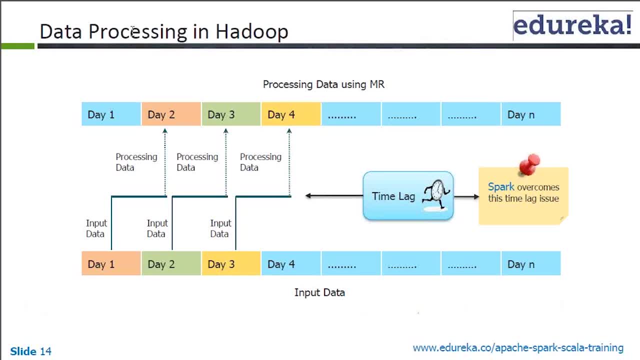 So I'm not saying this time lag is going to be zero, no, But this time lag is going to be much more manageable because there are some of the timelines which are acceptable to the business and then there are some which are not right. 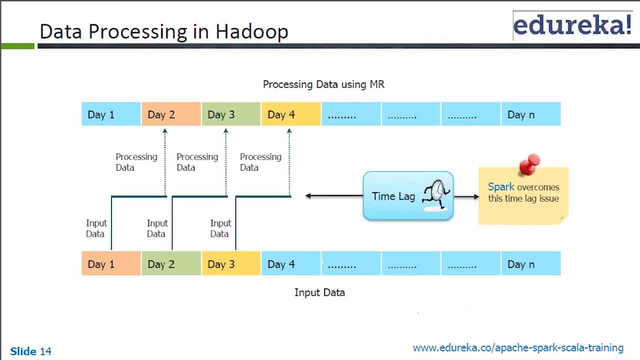 So in many cases we have seen as of now, I have implemented three projects in Spark. When I say three projects, it means in the, at the organization level, and one of them is going into production, one is in POC and another one is kind of in the ideation stage. 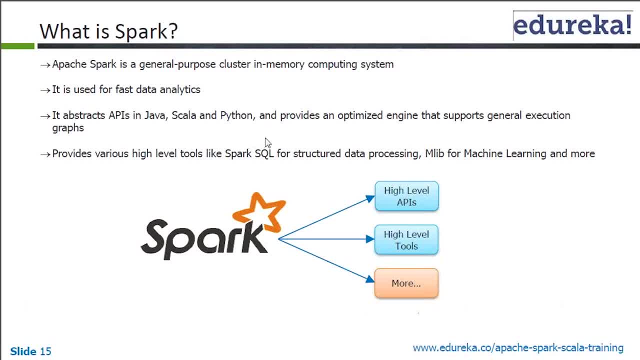 kind of Okay. So Sridhar says: when you say Spark plus Hadoop, is it integration of Spark with Hadoop? Yes, Sridhar, Okay, Spark again. this is again the slide which you must have seen earlier, I am sure. 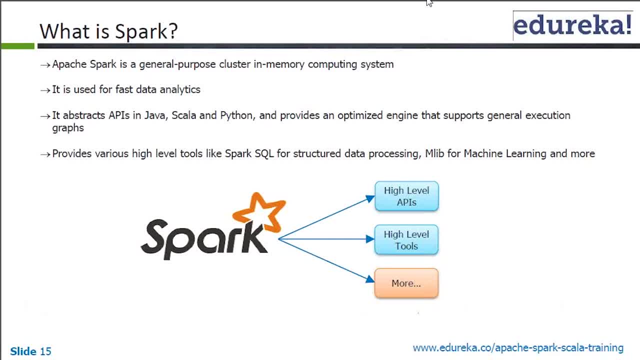 I hope everybody is able to recall, So I don't really want to spend much time on this slide. Or unless somebody wants me It's about, I had spent quite a lot of time when I told you that it is a general purpose cluster computing system. 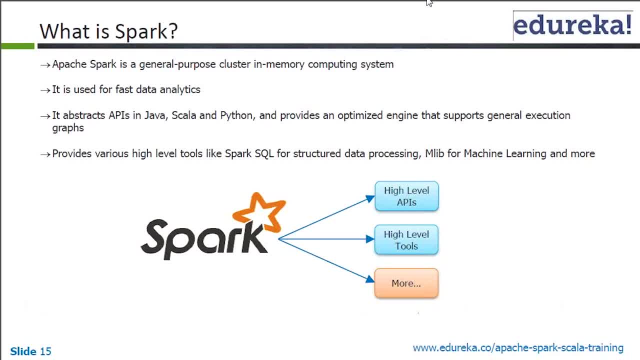 If you just look at this, it is Hadoop right General purpose cluster computing system, But when you put in memory then it becomes Spark. So it's a general purpose cluster in memory computing system. The computations happen in memory rather than streaming the data. 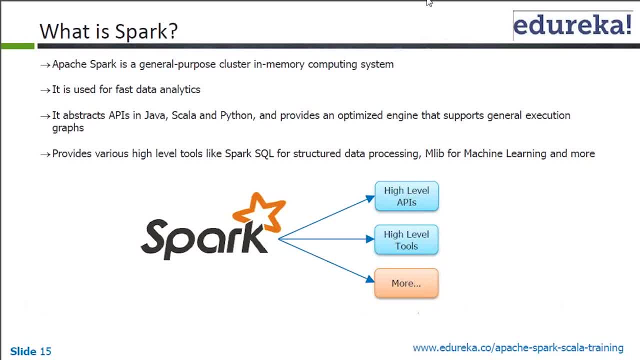 The data from the disk itself. Is that clear? And it is used for fast data analytics. blah, blah, blah. whatever about these high level tools and all These are some of the things I am sure you are able to recall. Does anybody need any explanation on any point here? 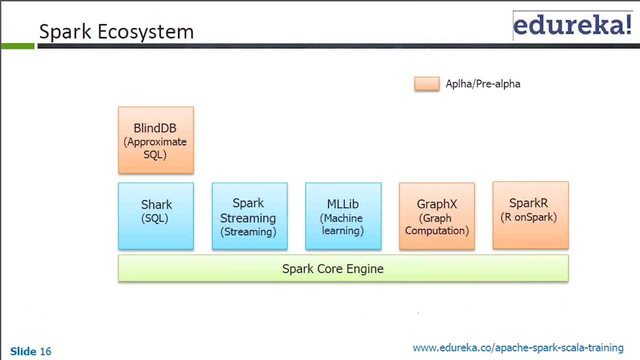 If not, I am moving to the. you know some more important parts. Okay, So spelling mistake: It is Blink Blink. What is blink? DB guys? I am so sorry. I have to inform the support team. It should be blink. 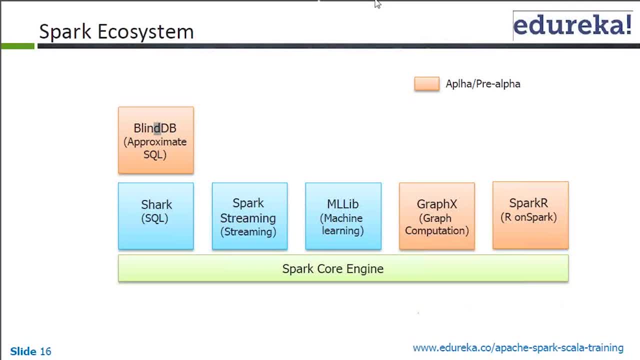 DB. It is not blind DB. So now this is Spark ecosystem and you can see that many of these releases are in alpha or pre-alpha releases. It means they are not even available for kind of you know, exploring. So Spark is not available. Graphics is almost unusable, It is kind of 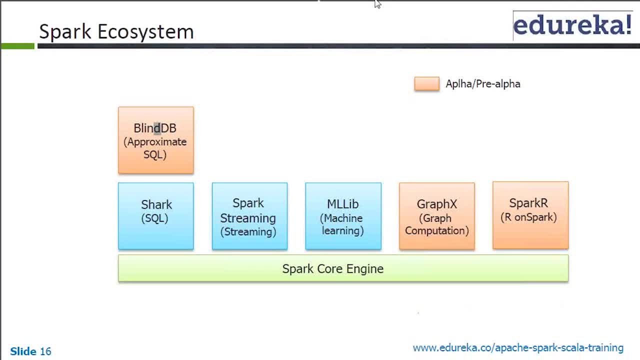 they have recently released an alpha release, but it is a bit unstable with the latest one. The things which are kind of you know are Spark Core Engine. Yes, it works. You can write your core Spark programs. Very good, ML Live. There are some of the things which 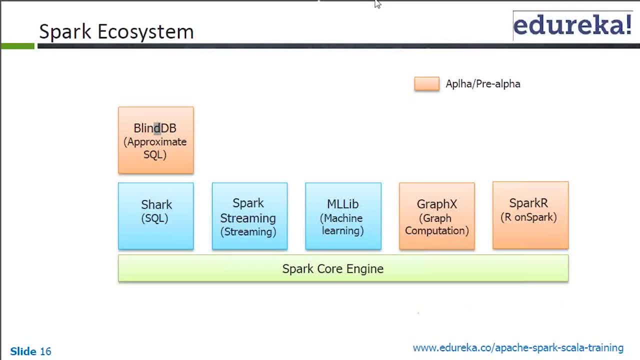 have just come up And you have the shark which is basically: you will be using the Spark engine. You can write your core Spark programs. Very good, ML Live. There are some of the things which have just come up And you have the shark which is basically: 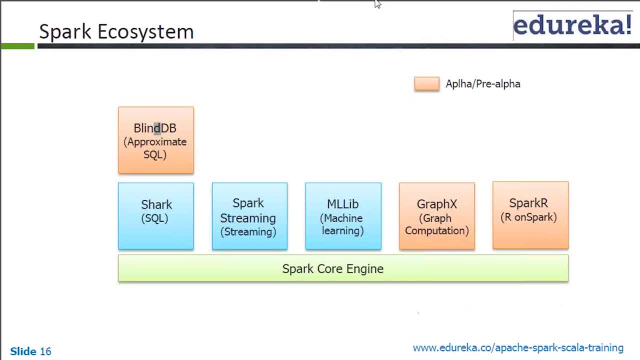 using for again, I have covered these things. That is why I am not spending that much time right now. It is about you know shark SQL for the SQL thing, Spark SQL. So shark slash Spark SQL. you can say that Shark is something which is full-fledged available Spark SQL. 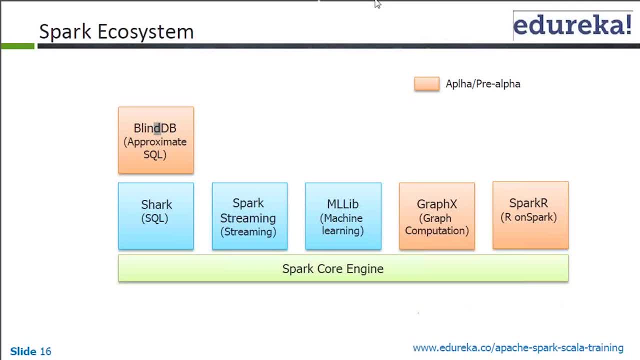 is something which will be available after you know sometime in the full-fledged manner. Right now it is about you can expose some of the documents in the form of some tables, but not really the hype tables as such. Okay, And then you have Spark streaming. We will be seeing that example. You know Spark streaming. 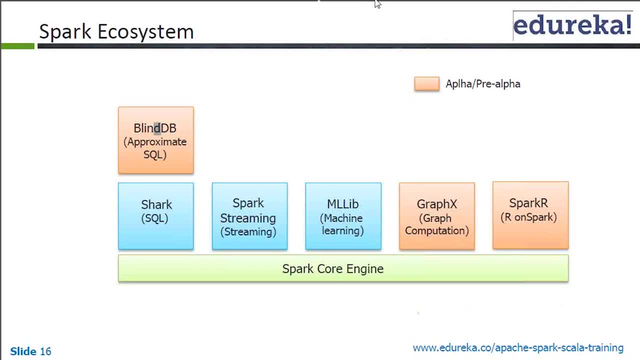 ML Live. So instead of spending time on ML Live, I have kind of created- I am not really sure, It is somewhere in between of the first batch and the second batch. I am trying to create my own machine learning, small kind of you know experiment, And I am somewhere. 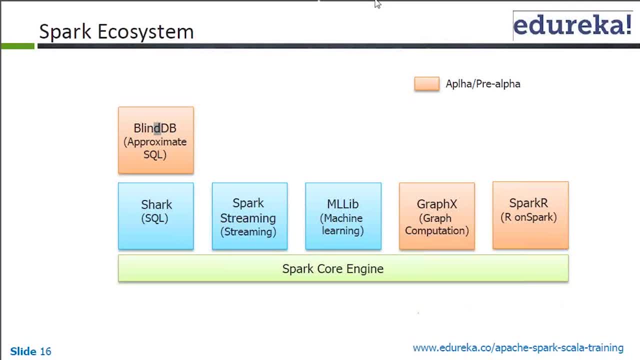 in between, guys. I am not really sure how to complete it and all. It is somewhere in between. But yes, it is about How to perform data visualization using Spark. I am working on that. So, if you have some data, how do you- you know- approach about it? How do you really show in the form of graphs? 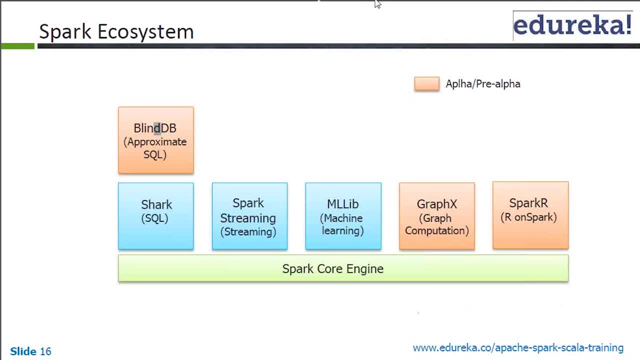 and all? Will it be exciting for you to look at it? Does it excite you enough? Or it is like, okay, we can look at it later, or something like that, Because I am planning to show it in the class. That is kind of the advanced stuff which I am just trying to achieve. Okay, 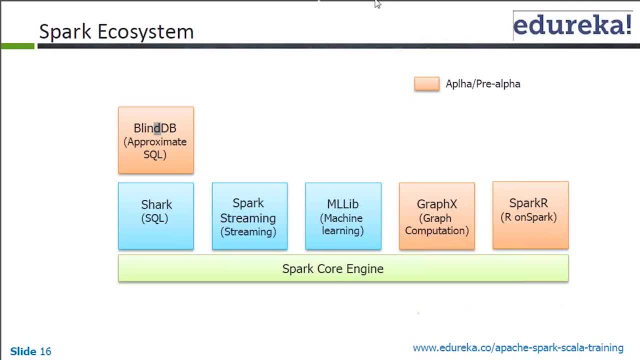 And since, great, And since, when it comes to the you know, graph graphing and other stuff, R Spark is not yet available And Scala does not have a really good you know that histogram and other other thing, other other capabilities, So I am using Python for it. Okay, So just. 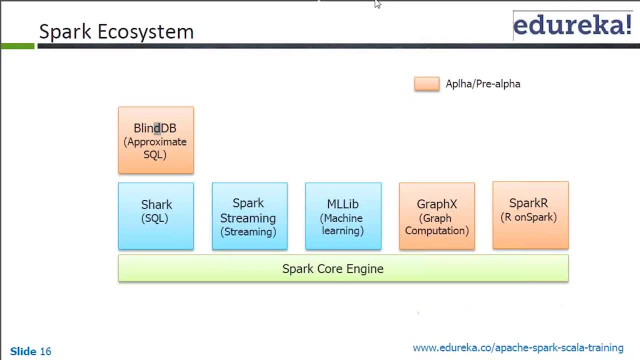 for that. you know I will be sharing, whatever I have done, That entire source code and data also with you people, But still you can take it forward. It is kind of I have to do some more work and then it will become up an application itself. Okay, So I will be trying to show. 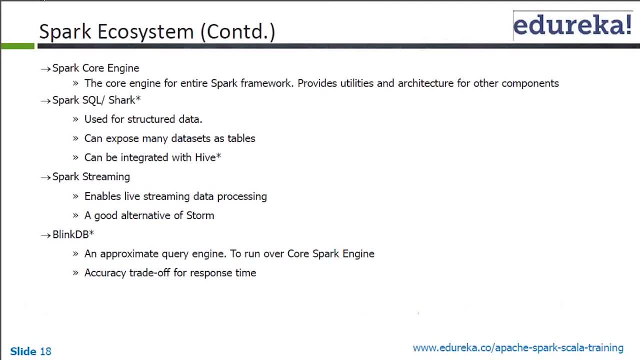 you some of those aspects in the last class. Okay, So again when it comes to the Spark ecosystem, again this is something which is already well discussed, Right? So Shark is basically Shark or Spark SQL for SQL kind of you know analysis, And they are typically 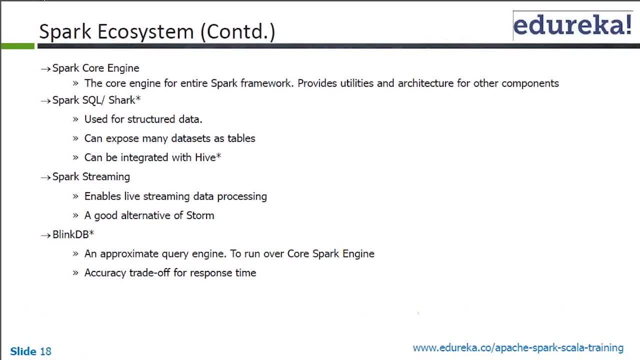 called data science tools, Right. So you want to perform some sort of analysis. So if you want to perform some sort of ad hoc analysis, you would like to use Shark or Spark SQL or even BlinkDB whenever it will be available- Right. But if you are more of a developer, 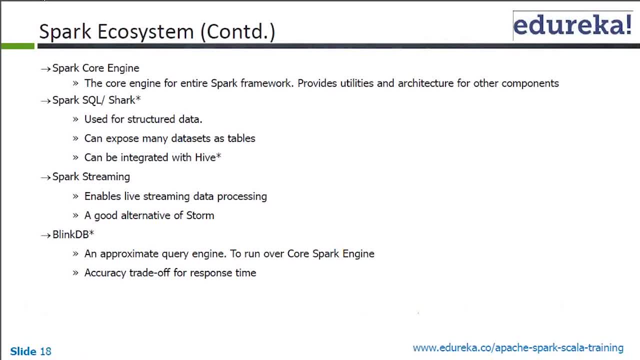 kind of a person, Right? Your, your job profile is more of a developer kind of a thing. Then you would typically like to go for Spark core engine, use Spark streaming or ML live when it will become mature and all Right. So these are some of the things which you will. 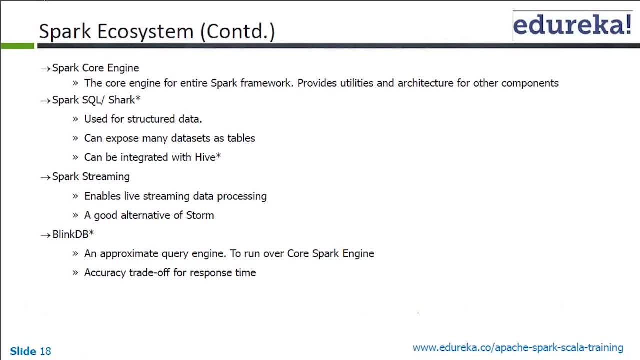 be using And in fact, guys, since Spark is a very fast moving community in, for example, if you want to further some more iterations, you will see some of the, you know, new modules which will be added. Okay, This is my plan To add some new modules as and when these 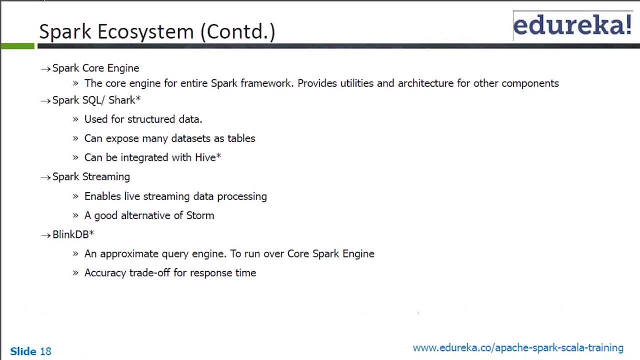 new things will become available. So, and anyway, since you have the LMS access for lifetime, you will be seeing those additional things for yourself. So it is just a request: Keep watching them. Okay, Once the course is over, at least you know whatever will. 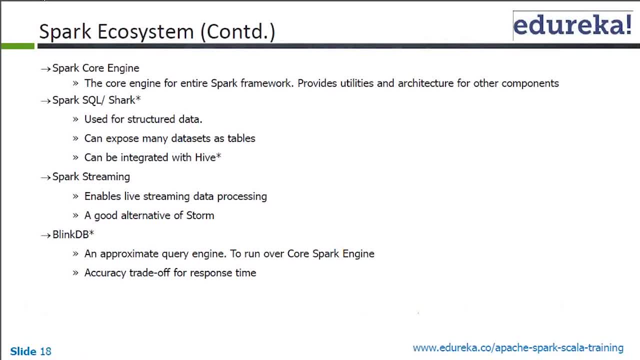 be the updated version or material. it will be available, I think, with the recording. okay, So this is just for your vision, Right. Bit more details about basically. there are some other aspects which I want to cover. Is everybody okay with it? Spark core engine. Spark SQL. 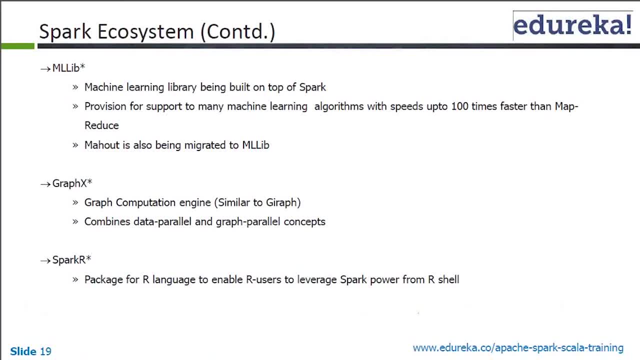 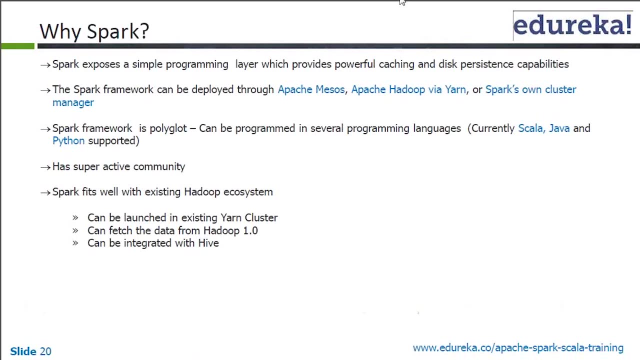 shark. we have already discussed this, Right? guys. ML live graphics, Spark R- what exactly? they are Right, So I am not spending the time on it, I am spending the time on which is important. Okay, Now, this was kind of you know, just in case if you have forgotten, guys, there are some. 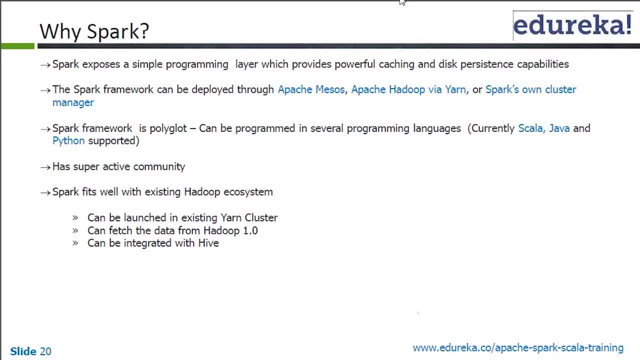 important things about why exactly we should go for Spark and all again. So these are. apart from that, Spark ecosystem is providing you various tools to do the things. there are some other things which are important or which are present in your application, and that's the end of the session. Bye for today. 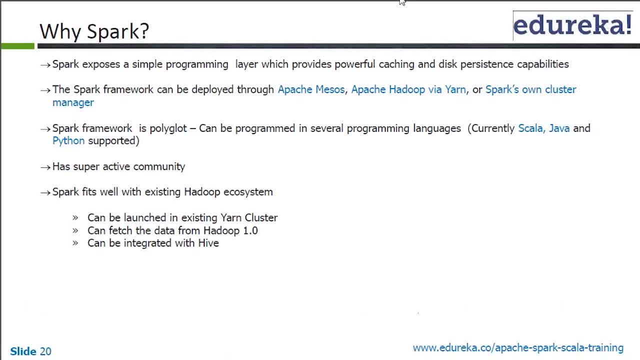 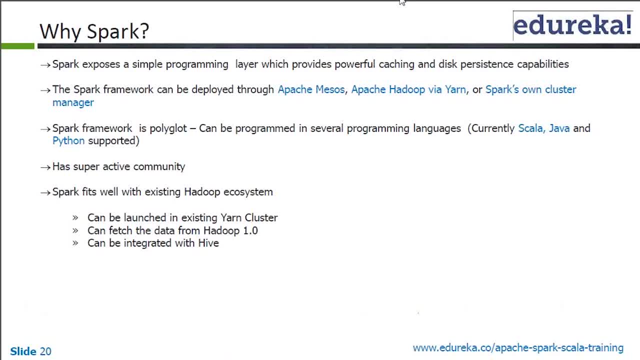 it's not just a programming layer. it's about its caching capabilities and this persistence capabilities. you will see that when I will talk about RDDs- right, resilient, distributed data sets- when I will talk about that, you will see these aspects in action. okay, so, caching capabilities: you can cache the results. 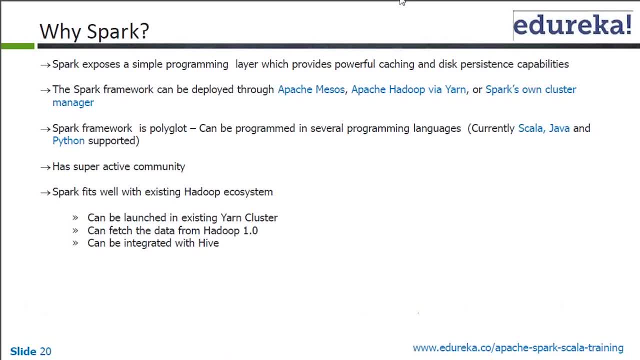 if they are more than this much, you know, more than a certain number whatever, or more than a certain limit, then you can either persist them in this fully, partially, up to a certain factor, and things like that. okay, so there are some of the factors which are available, and other thing is spark is something which 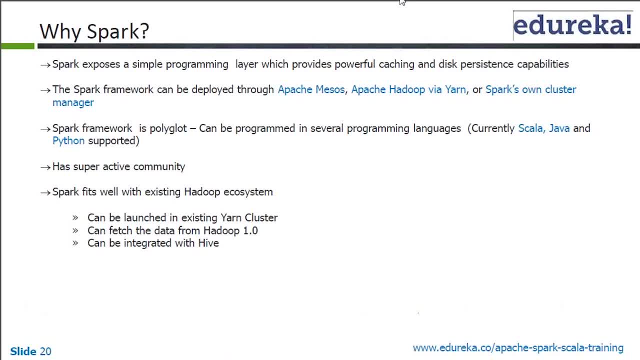 is not a very tightly bounded kind of a system. so if you so, if you have, let's say, your own. basically you are running spark in a standalone mode, right? no other cluster manager, it has got its own customer manager. but otherwise you can integrate it with yarn, which I will cover in the 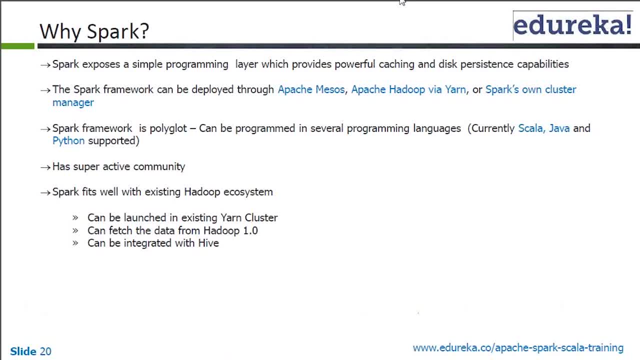 class and with mesos as well. mesos is something which we do not cover, but yes, it can be, you know, integrated with it as well. okay, it's polyglot. I have just told you Scala. you have just seen Python. you can write the programs in Python as. 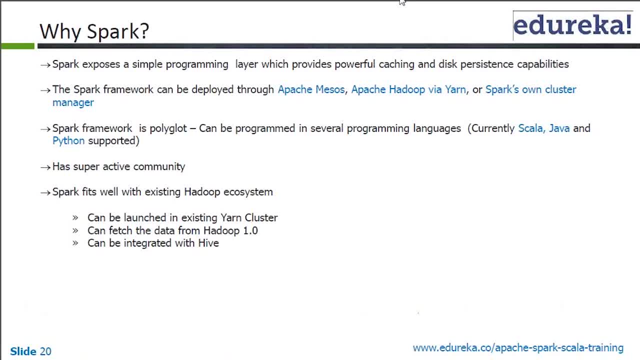 well, and Java also okay. it has got a super active community and all completely okay. it fits well with existing Hadoop ecosystem. now, guys, this is very important. can you look at this second point before the first one? the second point which says it can fetch the data from Hadoop 1.0? right, this is very important. many. 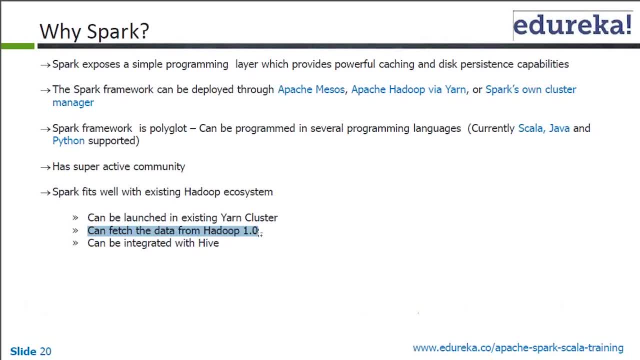 times I have talked about it and I have talked to many people. they say that okay, if you have to use a spark with Hadoop, you have to use Hadoop 2.0. okay, you have to use it with Hadoop 2.0. no here. 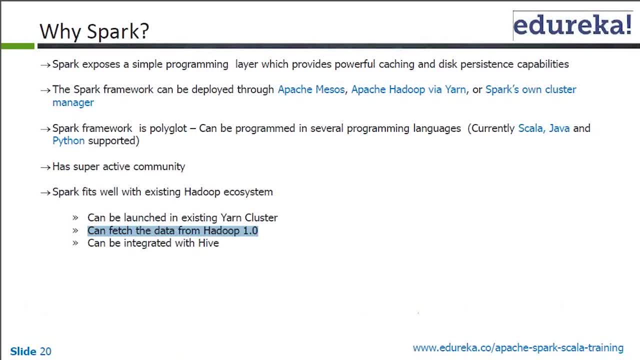 it can fetch the data from 1.0 itself. but remember, you are just fetching the data. you are using Hadoop as the storage. you are not using Hadoop, the cluster manager. if you are using Hadoop as a cluster manager, then the first line is: 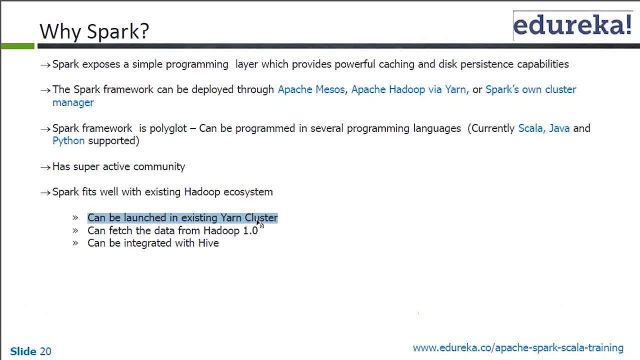 very important. it can be launched in the existing yarn cluster itself- okay, if you really want to use it. and of course, it can be integrated with hive. of course I the in the bracket. it goes without saying that right now using shark, in future using spark SQL as well. so 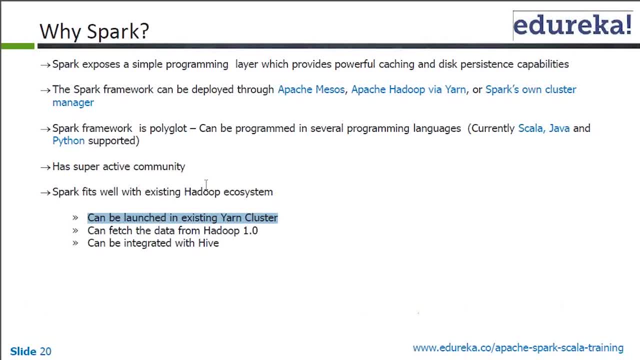 this is how it fits into it. by the way, as my experience says, most of the times it would be the second use case which wherein you would like to use it. you would like to leverage Hadoop's storage power more than its processing power. we will come to that, Lakshman says. 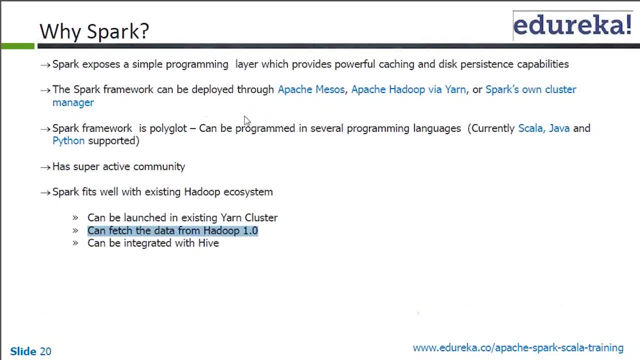 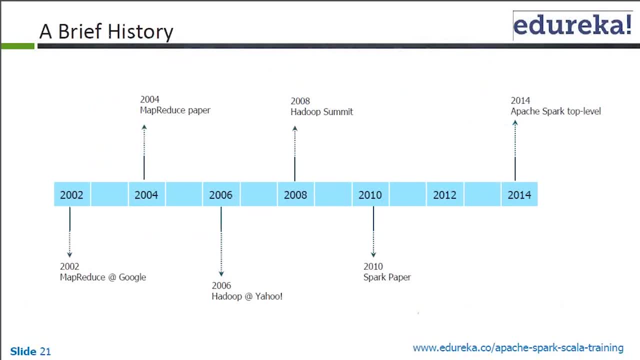 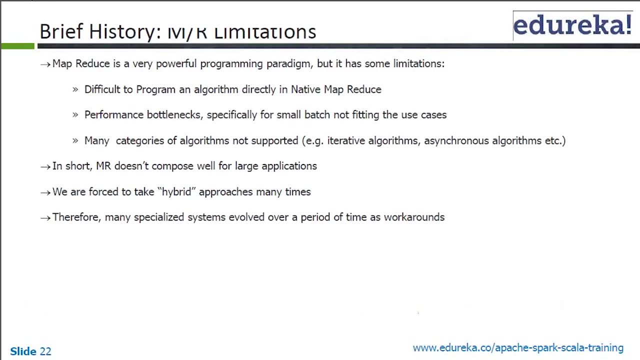 something I had a very bad experience with in memory tools click view when RAM maxed out. I am not sure how spark handles it. yeah, Lakshman, I am coming to that part. so just a second. let me see how much we can cover. in fact, we are already at 10.15. 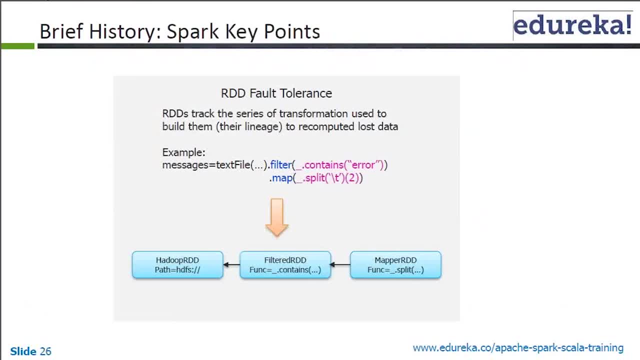 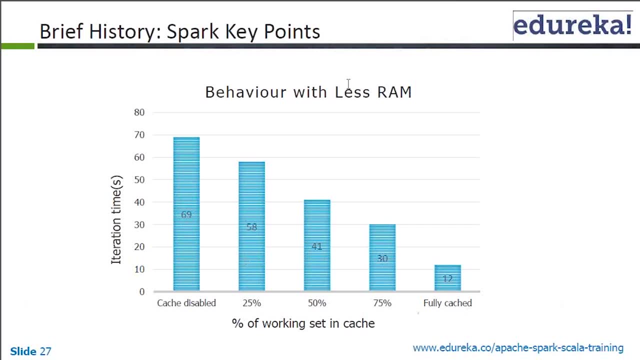 ok. so Lakshman, just to give you an answer, say this: ok, so this is the execution time and this is the percentage of working data set in the cache. if you fully cache it, this is going to be your response time, let's say 12 seconds or 12 milliseconds. 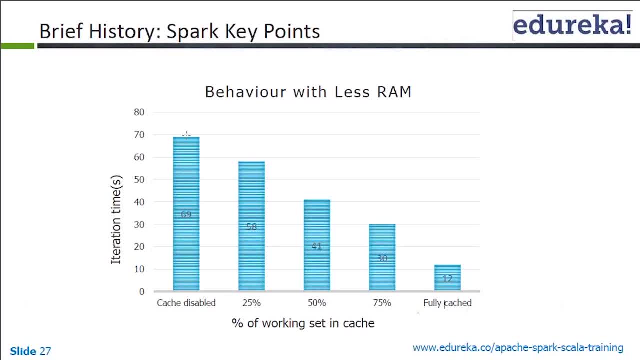 and if your cache is disabled, this is going to be 69 in between. it's a graceful degradation. I will cover that more in the next class, tomorrow's class right, Lakshman, but it should just give you an idea about it. 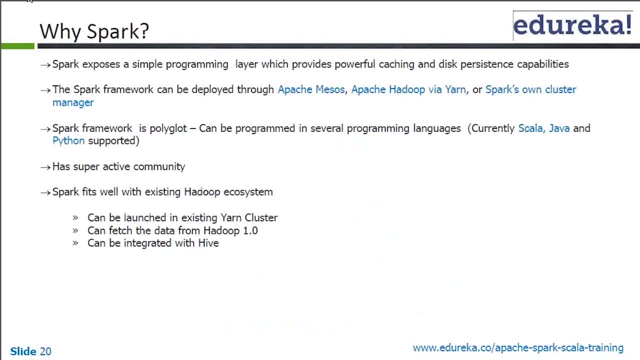 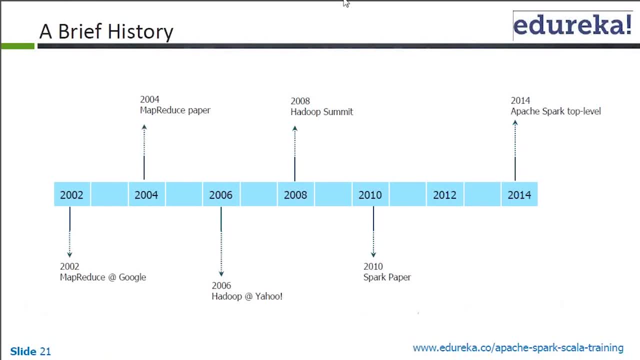 right. so, guys, I think it's. I should not extend it, you know, any further. I will just cover this slide, number 21, and then we will just continue on the things tomorrow, right? so about history. again, it's just a theoretical point. 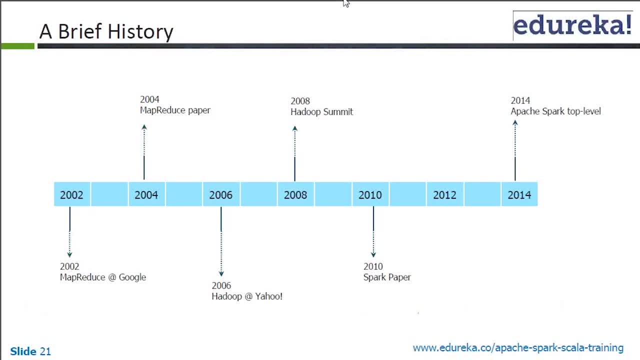 all. I am not spending much time because you can read it, the. I am not spending much time because you can read it the point first that makes sense for me to explain. eh, don't catch up on it, it is soccer acronym, because the name of that game is just basketball. 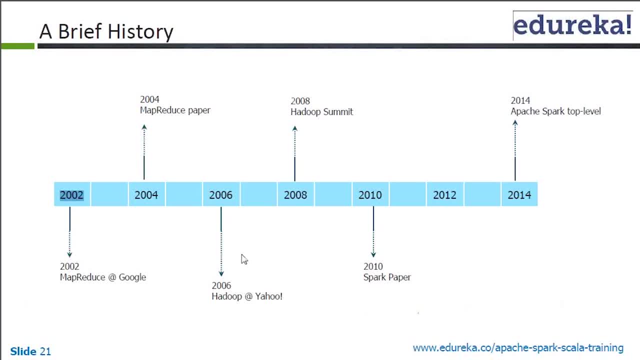 before you watch the video, isサンデرا. you already knew how to play soccer till the very end. what. what does it mean? you must know, or you must know, how to use it. then, at the bottom square, at that pointI will write down the names and the names themselves. 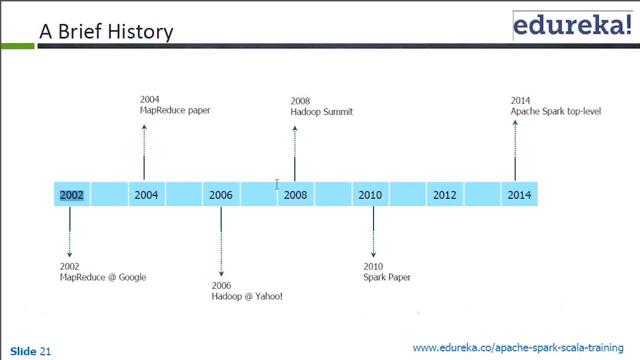 so at that pointwhich I want to say is 2000 forma, six years. it took six years, which is kind of a defective standard, right? I hope everybody understands it. 2010, spark paper got published. it was, it just got published. 2012,: it was: 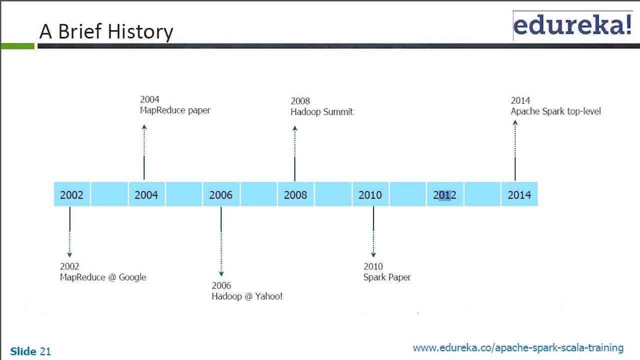 actually adopted. it was adopted means it was its first implementation came out. first implementation came out in 2012,. okay, and it was not a Apache, and it was 2012 late or 2013 early. I have just forgotten when it got adopted by Apache as an incubator project. 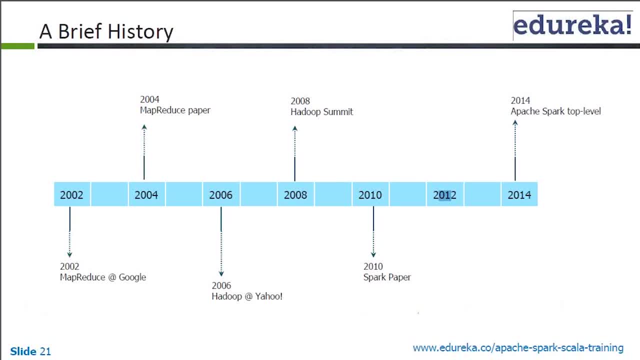 okay, we are just talking only one year early, kind of one and a half years earlier, okay, and right now it has become top level Apache project. Just look at the: this is the first project which is the fastest to achieve top level status in Apache. okay, and it is. 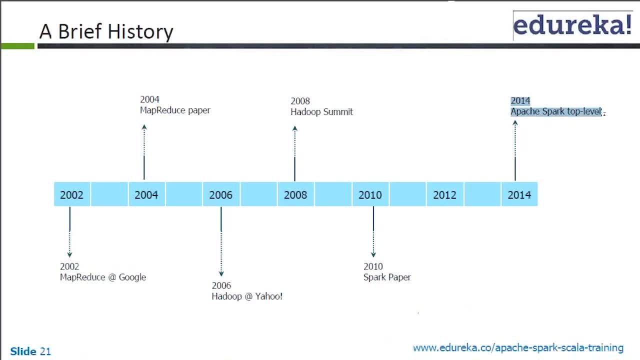 coming up big time. why? why it is not just that everybody has heard about spark and everybody is putting the effort right. Cloudera is betting big on it. Hortonworks is now betting big on it. right, for a reason, right? so for those reasons, right, Devendra exactly. 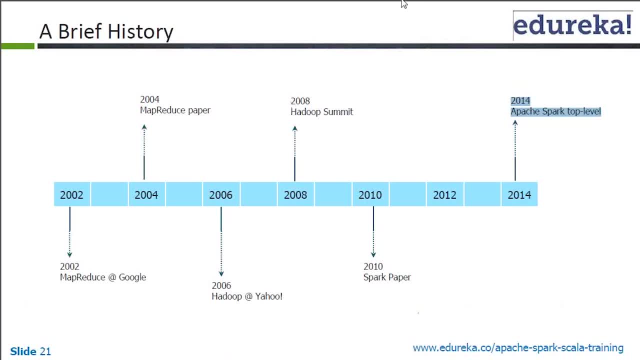 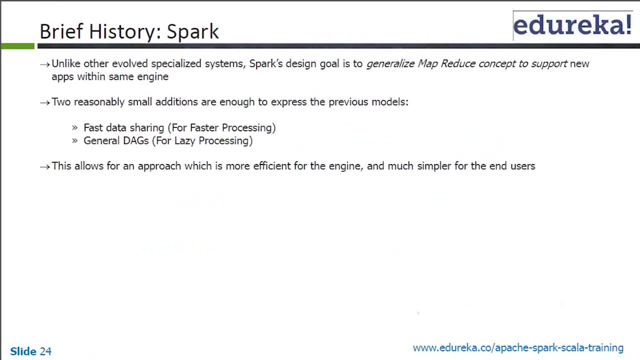 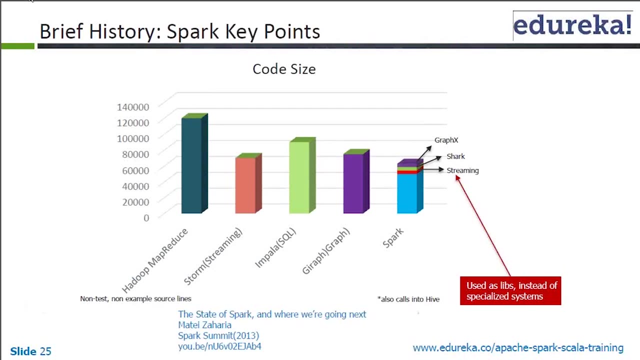 Devendra, the question which you have asked, right, how do spark and storm compare? all I would say is you will get the answers from these slides: slide number 22,, 23,, 24, and 25,, basically up to slide number 26,. okay, 22 to 26 have the answers for your question. 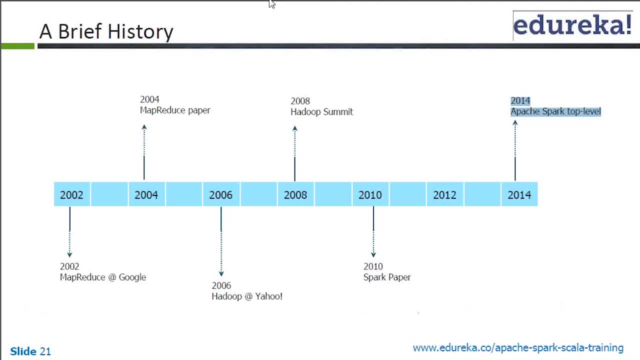 okay, Devendra, I will remember your question. you will get the answer if you do not. if you do not, then I will tell you. Okay, so guys, I think yes, this is where it is. I hope it is good to give a logical. 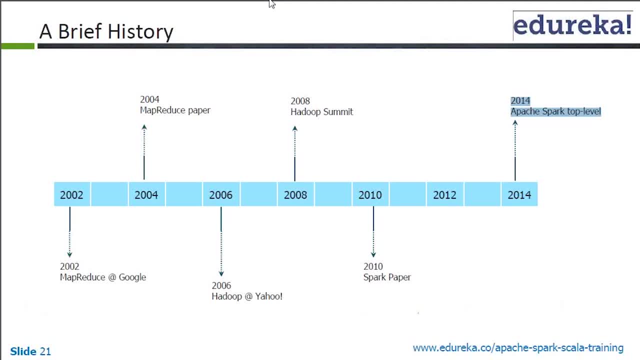 break and see you then tomorrow, and I hope you liked it. we made quite a good of progress. I mean, if you see, it is slide number 21, where we are, it is not really slide number, slide numbers which matter to us, right, because there would be two or three slides. 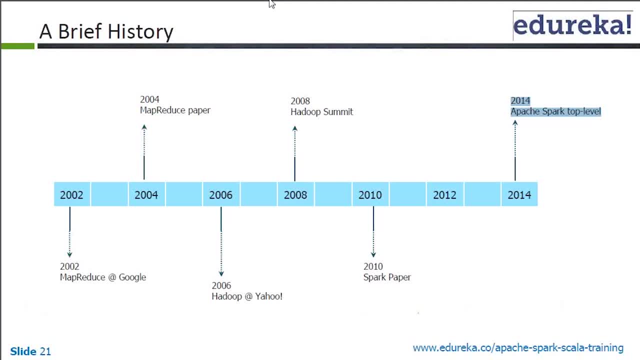 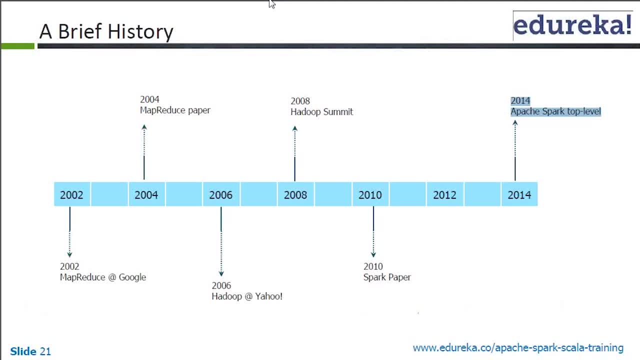 you know, just pass them through, right. so tomorrow, tomorrow the session when it would start, there would be some serious topics about it. right that? how spark is different. as Devendra was asking question, storm versus right when not to use spark, right? so these 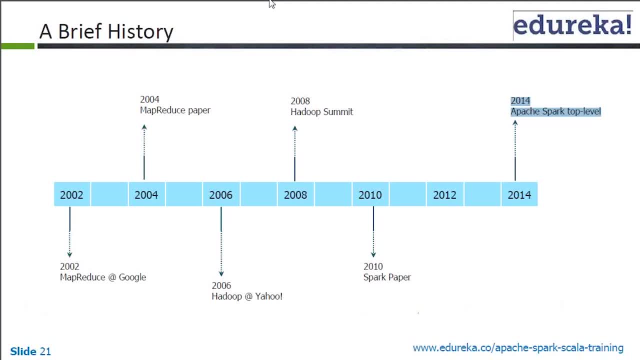 kind of things would come up. and then, immediately after that, I- since it is theory- I just want to finish it fast, and then I want to spend more time on the hands-on. Okay, So, Kalpana, just to avoid those. you know, within class people try to follow, and then 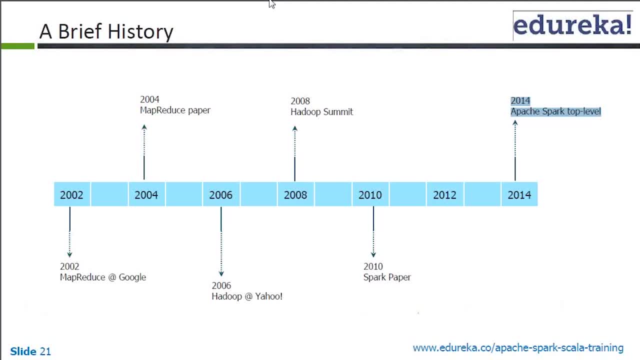 some- sometimes people don't have a good connection, some people get it delayed and all that's the reason we, due to which we have created the installation manual. okay, that installation manual gives screenshot by screenshot steps, But if you get stuck at any point, you can come back to me. I can answer. 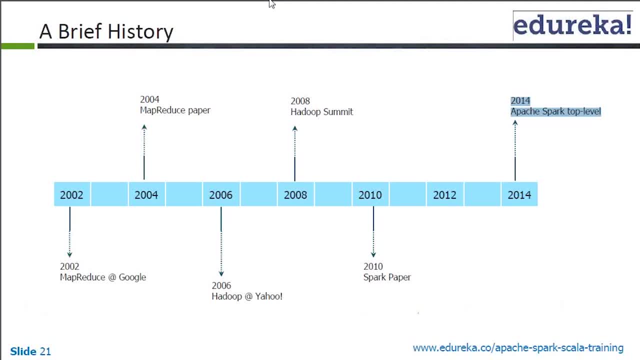 So you are supposed to do it. I will still try to go through them, not a problem. And you had question so I will. yes, yes, definitely help. desk will help in the installation and I think they must have helped one or two people. they will remotely log in and help. 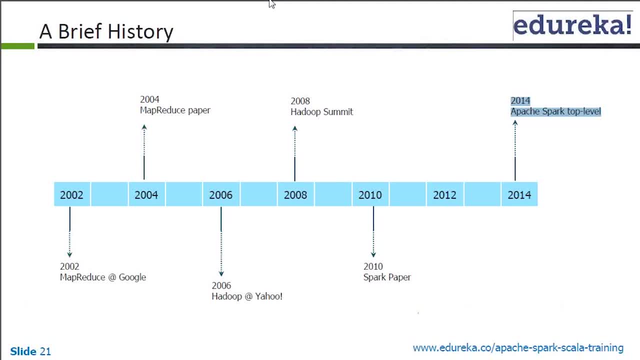 they must have helped you right, or somebody else, I don't know. So they have helped you there. Kalpana guys, do provide your feedback. that is equally important for us, please. So I always request for it, because it gives me the chance to see if there is anybody whose. 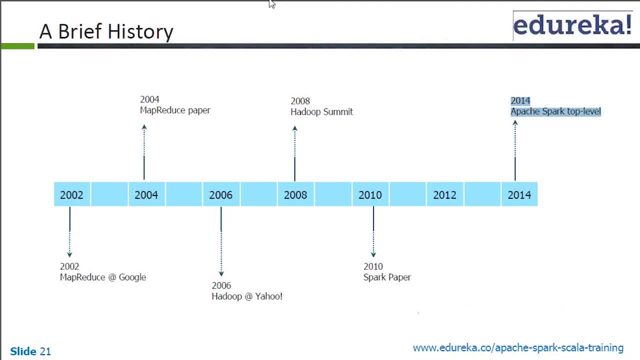 specific concerns are there which I can improve for that particular person? So, Raj, I didn't really get a chance to look at it. I saw it. I saw one mail from Raj, So I think it was you. I will just check it or I will just ask the support team to get in touch with you. 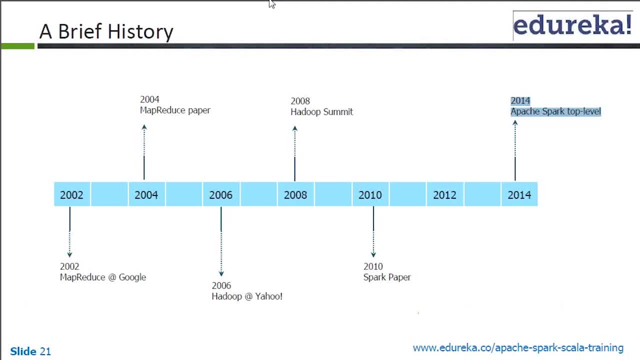 And don't worry, it will be solved, sure? So, Kalpana, if you want to ask the question now, probably you had some question which I said that I will be taking later. right, Others if you have. if you don't have a specific question, yes, I think we can discuss, for. 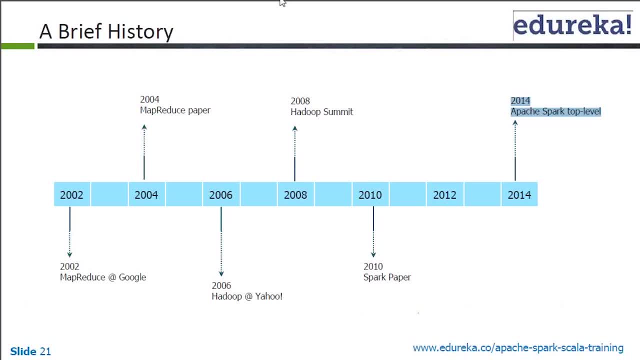 another day and you can, please, you know, do provide your feedback, guys. That's all I just want to say. Okay, Kalpana, you want to come on there. I won't be coming tomorrow due to personal reasons, but thanks, Raj sure.